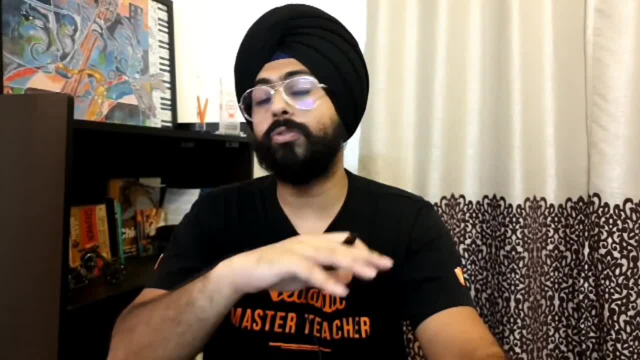 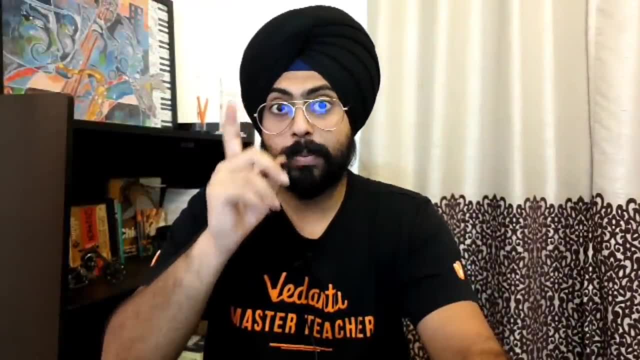 to discuss about chemical equilibrium chapter. This forms the basics of all the equilibrium, Yes, of all the different types of equilibria, And this is going to be a quick revision session, So please pay a lot of attention, Please focus, Let's get into it. So, my dear friends, 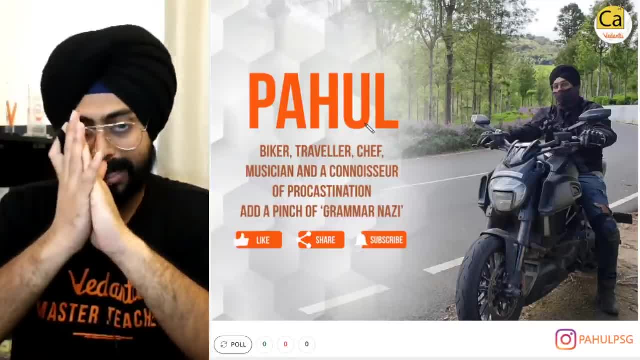 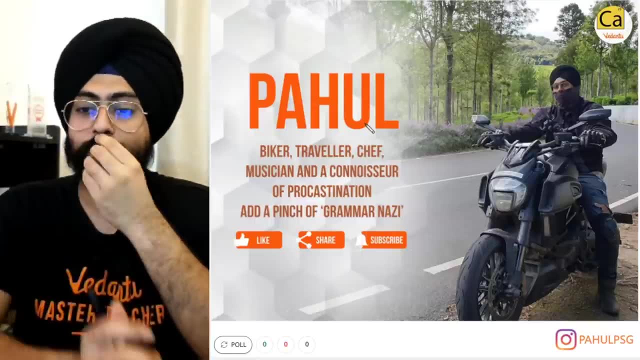 in case you are new to the channel, welcome to Catalysis by Vedantu. My name is Pahul and I am an alumnus of IIT, Bombay. I have lots of hobbies, as you can see on the screen, but I am not able to do biking and travelling because of this. 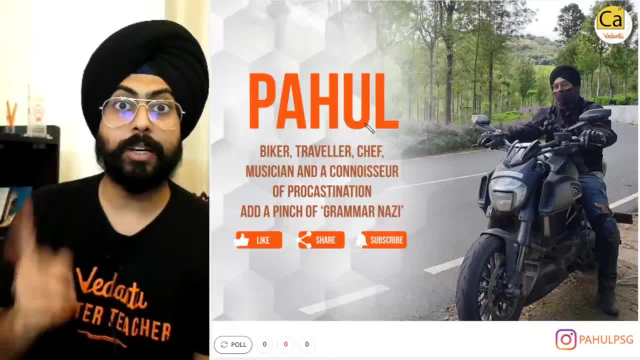 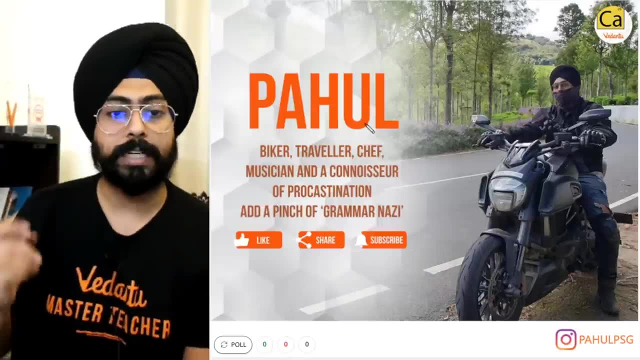 So are you guys ready to revise chemical equilibrium? It's a very small, very easy chapter, So it's going to be a very quick revision. Once the revision is done, we will chat with each other. Fine, Let's get into it. So, my dear friends, what is an equilibrium? 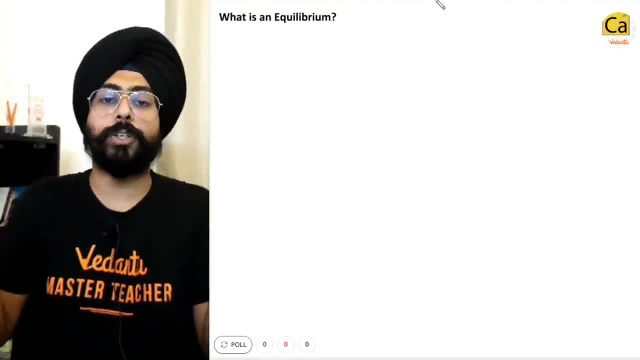 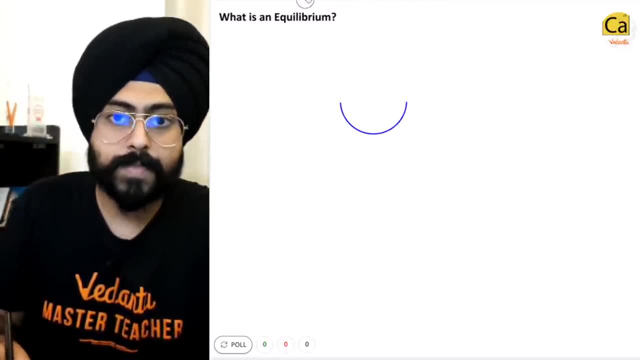 Equilibrium is a condition in which things are stable in nature. Yes, Whenever I think of equilibrium, I think of something like this. I think of something like this: where you have a tiny little ball, which is your body, And when you have a tiny little ball. 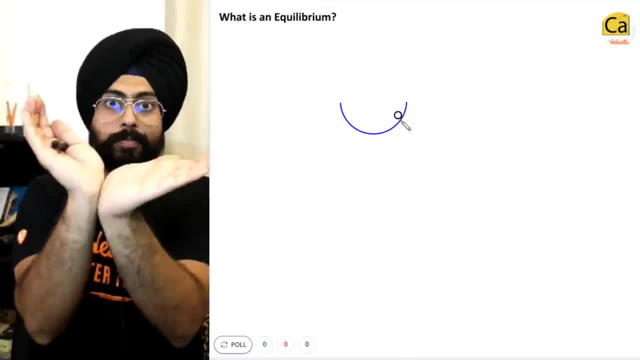 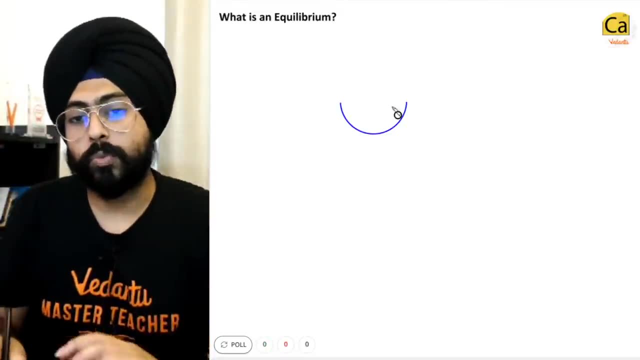 you know, sort of rotating around in this particular ball, And what happens is it will move around here and there, here and there and ultimately settle at the bottom. Yeah, So this is what comes to my mind whenever I think of an equilibrium, and this is what 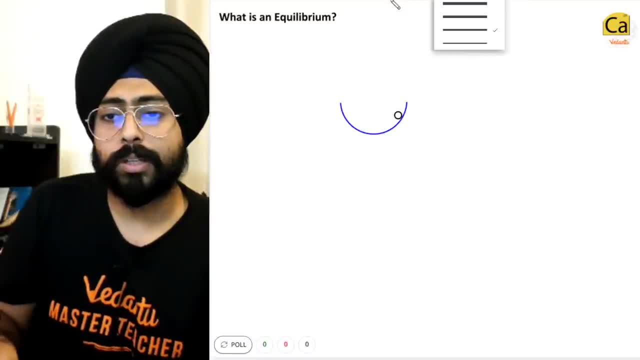 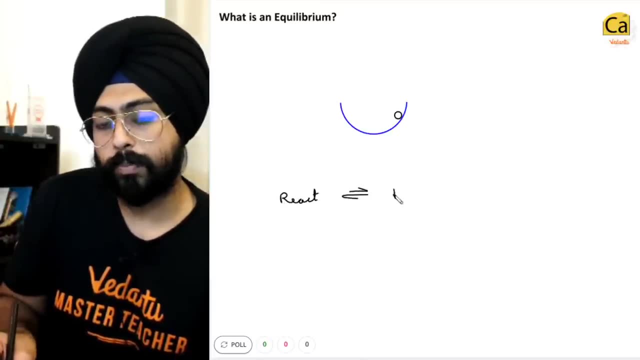 you also should think of Now talking about equilibrium in terms of a chemical reaction. Okay, In a chemical reaction, you have your reactants going towards the products And since this is a reversible reaction, the products are also going backwards. So you 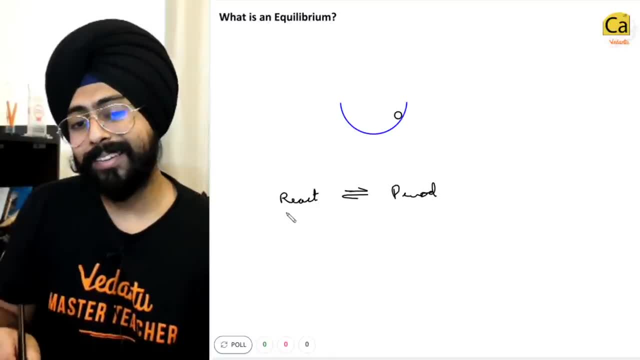 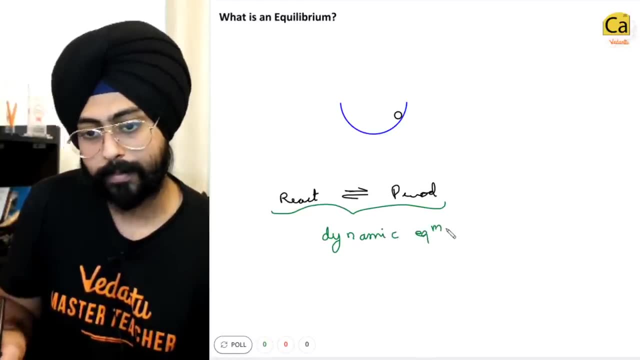 have the reactants going towards the reactants. So what's happening over here is: in case of a chemical equilibrium, you will have a dynamic equilibrium. Do you remember that? What is a dynamic equilibrium? Reactants are converting into products and products are. 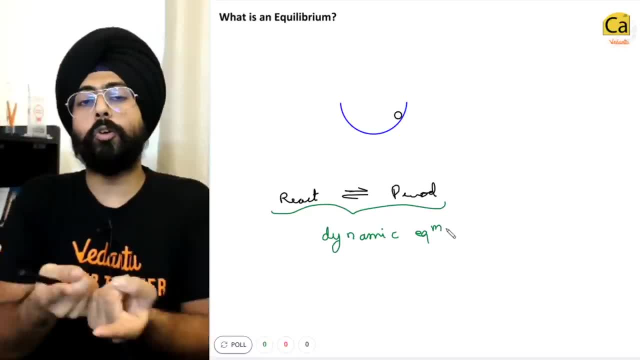 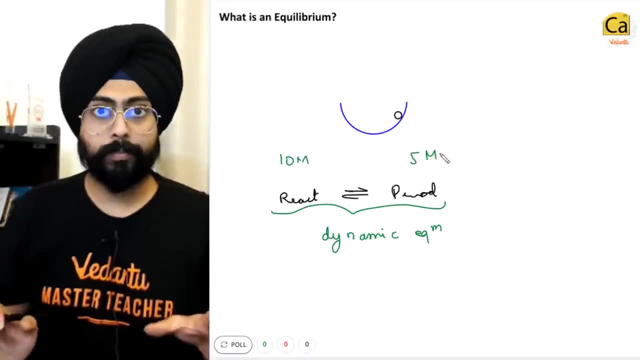 also getting converted into the reactants at the same time, But the overall concentrations are the same. Okay, So let's say you have ten moles of the reactants and five moles of the products at the equilibrium. This could be the equilibrium. Yes, Let's say you have. 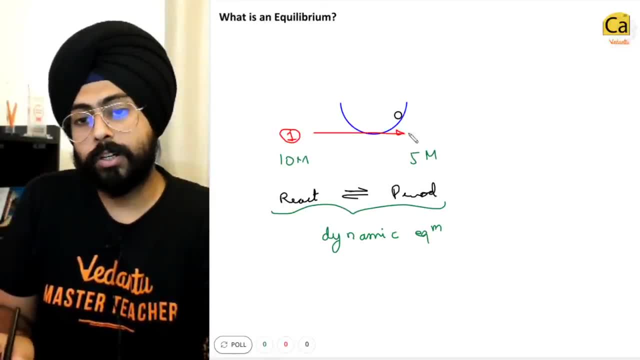 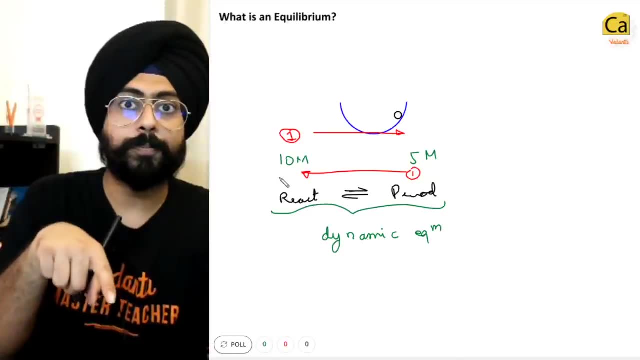 one of these moles gets converted to the product. what will be happening at the same time is one of the moles of the products will be converting into the reactants. this thing is going on, but the overall concentration of the reactants and products does not change. this is a dynamic. 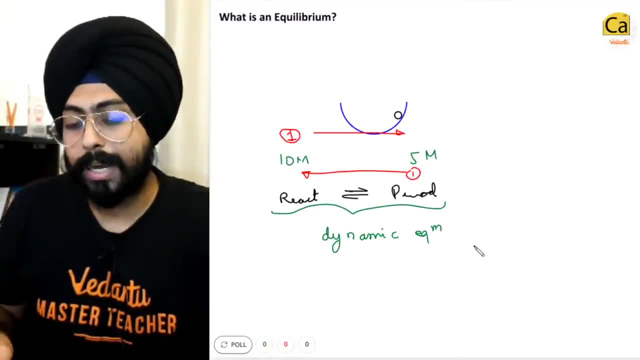 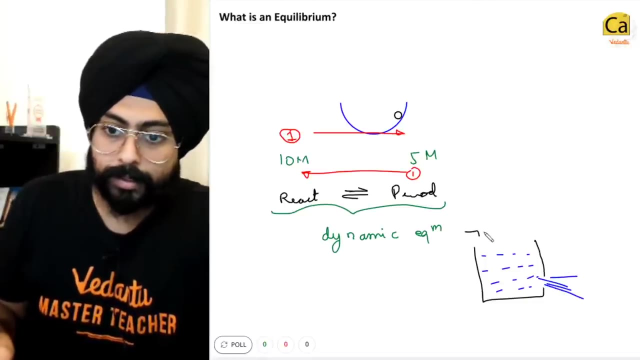 equilibrium. One more very simple example of a dynamic equilibrium could be this kind of a system where there is a hole in the bucket. there is a hole in the bucket, there is water inside the bucket, the water is flowing out of the bucket, but there is a tap on top of the bucket. 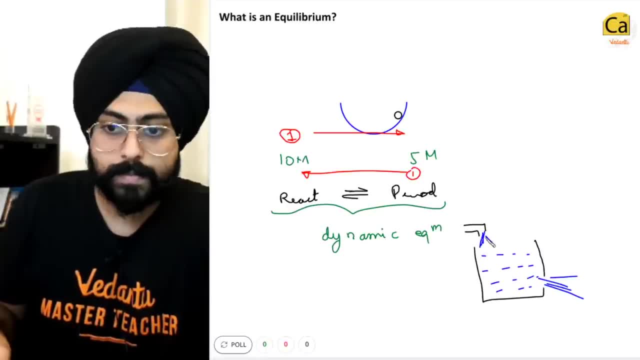 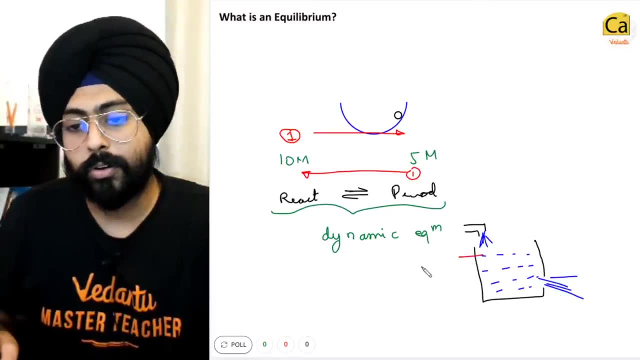 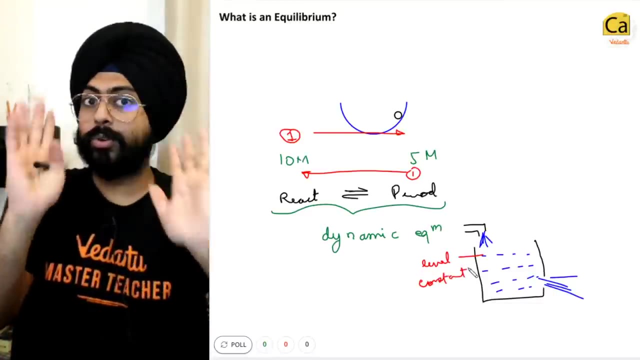 which is filling in water at the same time? do you realize that if the rate of incoming water is equal to the rate of outgoing water, the level of water will not change? level is constant, even though water is coming in, water is going out, but the level of water. 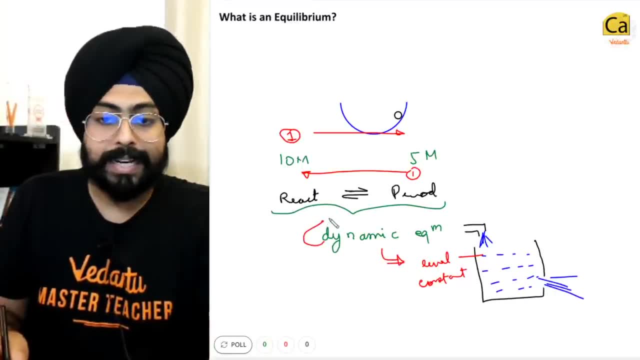 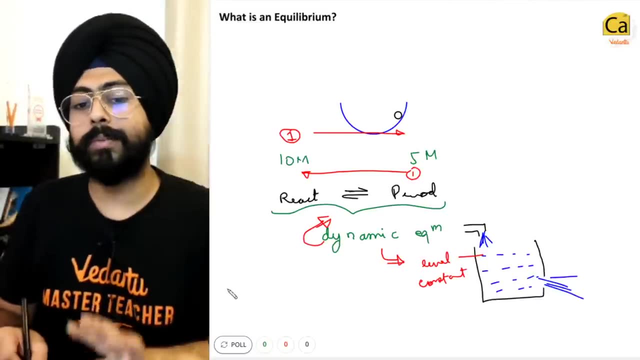 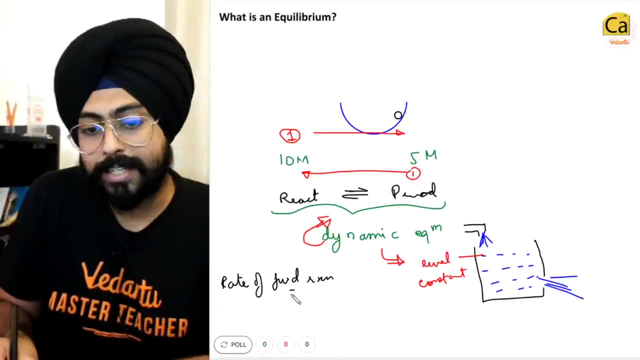 is constant. this type of an equilibrium is known as a dynamic equilibrium. So in reactants and products the same thing is happening, And in that dynamic equilibrium, one condition that we have to remember is that rate of forward reaction is equal to the rate of backward reaction, isn't it? 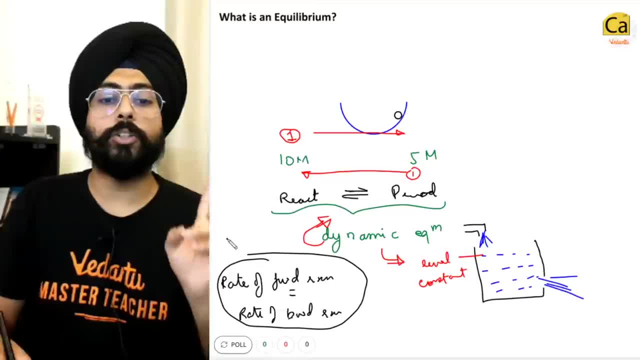 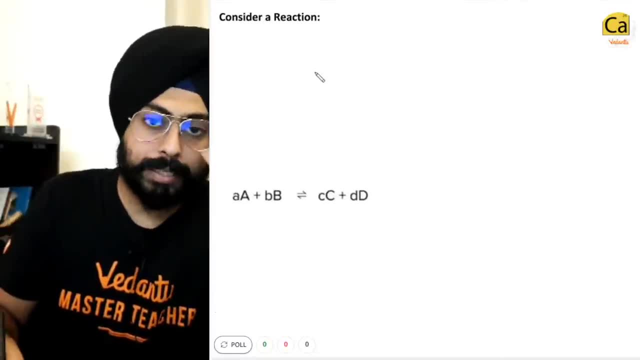 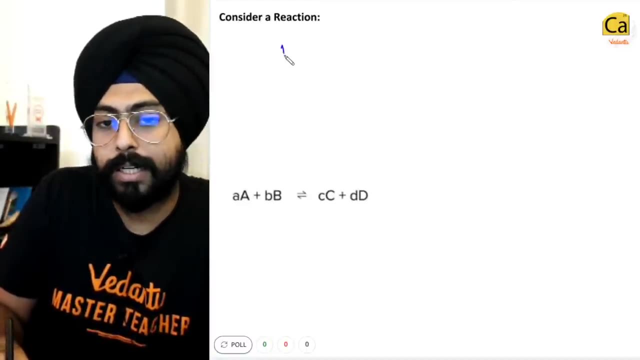 Rate of forward reaction equal to rate of backward reaction. this is the condition for chemical equilibrium. everyone knows that. Now, moving into an actual chemical reaction. So the reaction that I will take, For simple purposes, is this reaction which I always take. It is not really a chemistry reaction. I take one cheese, one slice of cheese plus two slices. 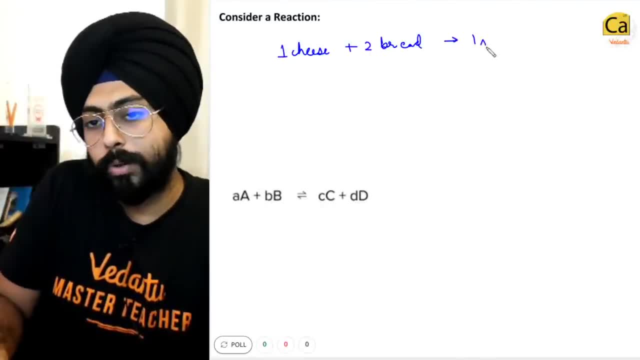 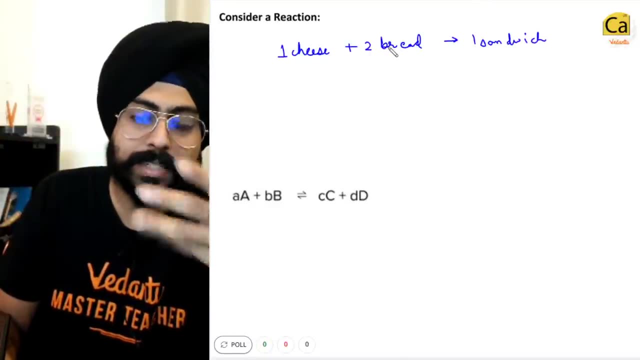 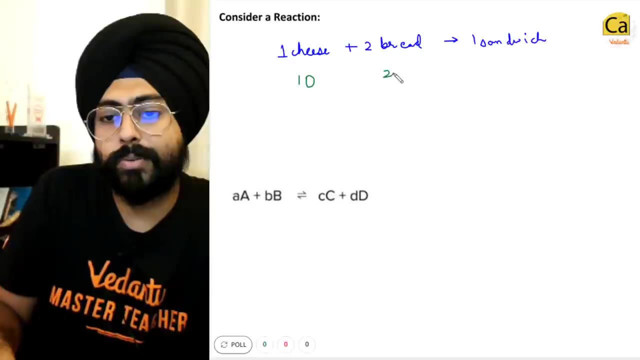 of bread gives me one sandwich. Whenever I teach reactions, this is what I take for an example. Let's say: this is the reaction. and let's say: you have 10 slices of cheese, you have 20 slices of bread, Whatever, so on and so forth. initially, 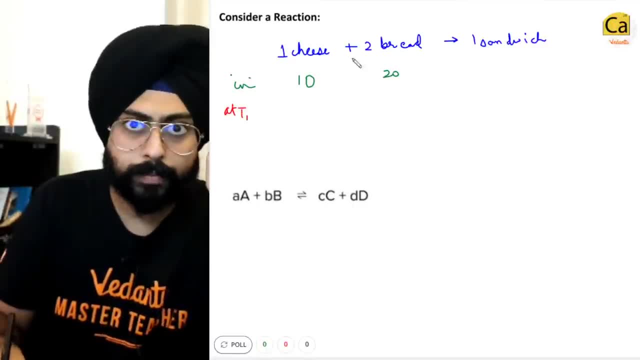 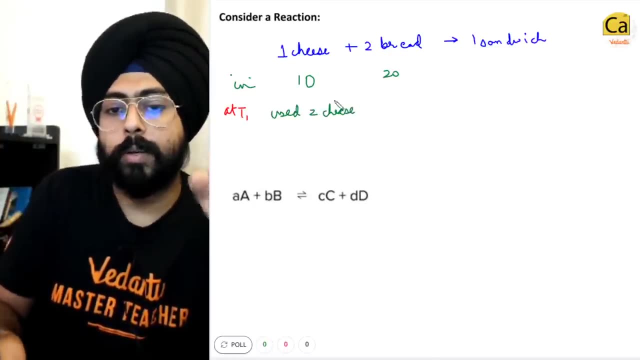 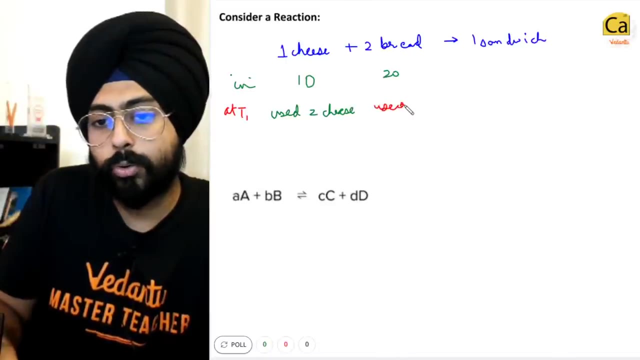 After some time- at time equal to t1, if I have used two cheese slices people, can you tell me how many bread slices have we used? agar do cheese slice use kar liya? so how many bread slices have we used? do you realize? we have used four bread slices over here and 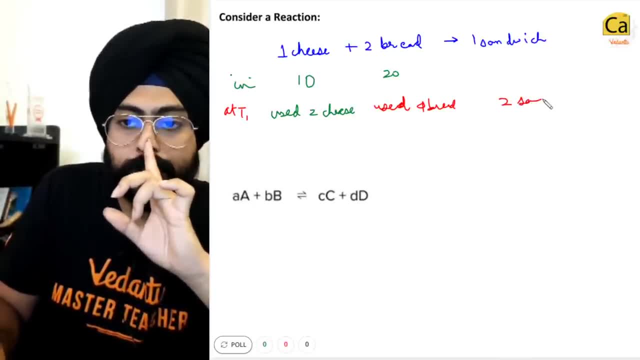 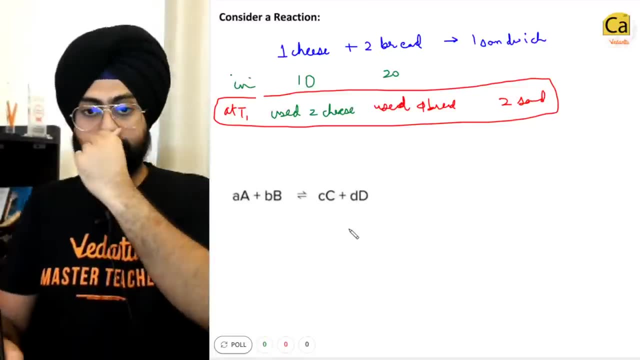 how many sandwiches have we created? We have created two sandwiches. So how many bread slices have we used At t equal to 1.. If this is the case, now my dear friends notice, I will write something and then try to fill in these values and tell me whether that's correct or not. 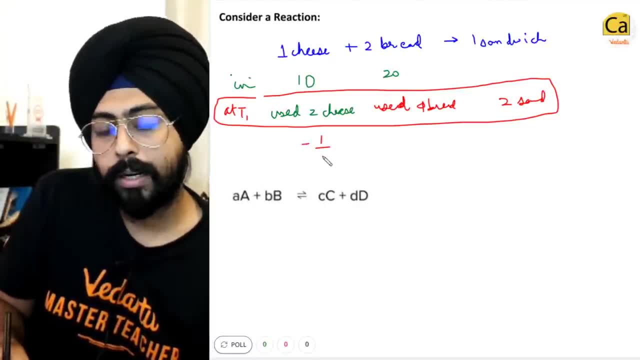 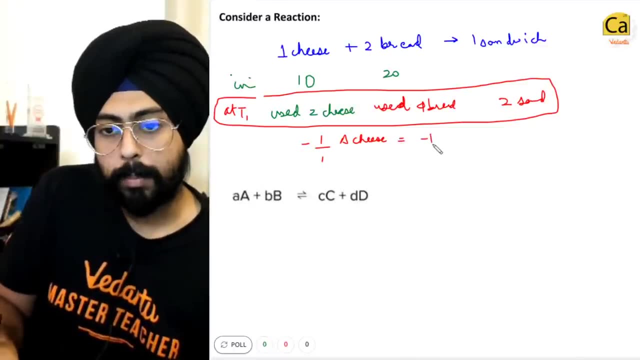 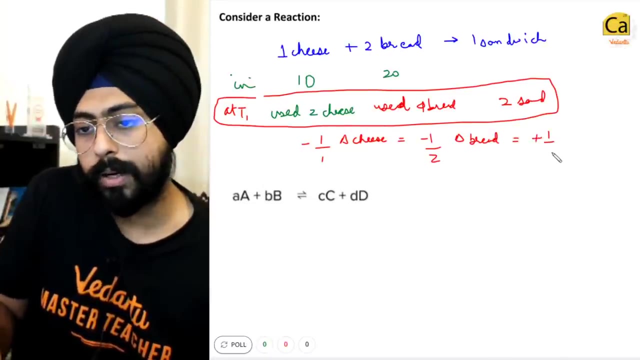 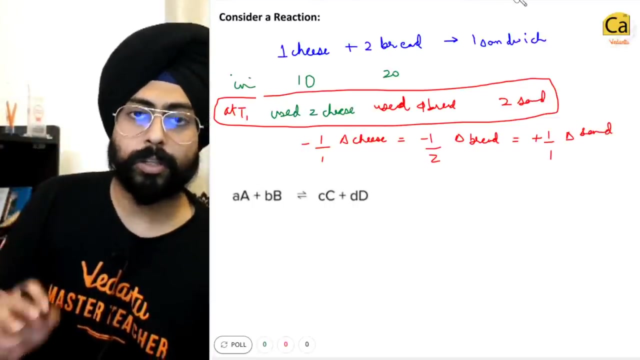 I can write: minus 1 by 1 times delta cheese is equal to minus 1 by 2 times delta of bread. it is equal to Plus 1 by 1 times delta of sandwich. Can I write this? My handwriting might not be the best, but I am pretty sure you are smart enough to understand. 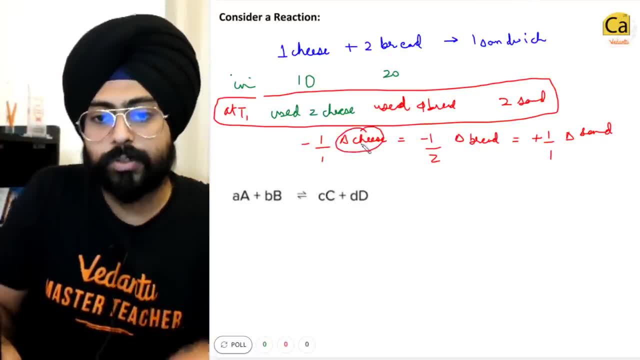 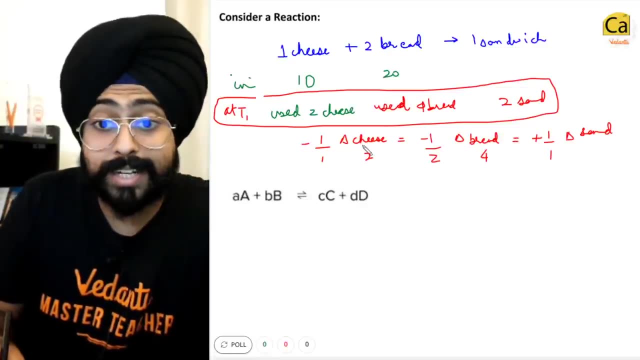 what I am writing. What is the change in cheese over here? Delta cheese is 2,, delta bread is 4,, delta sandwich is 2.. But do you realize that since cheese is decreasing, I will have to write minus 2.? 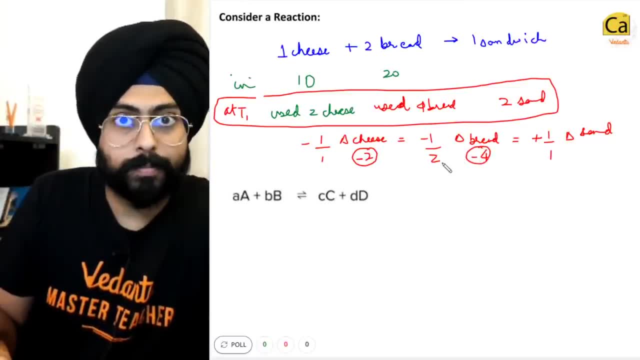 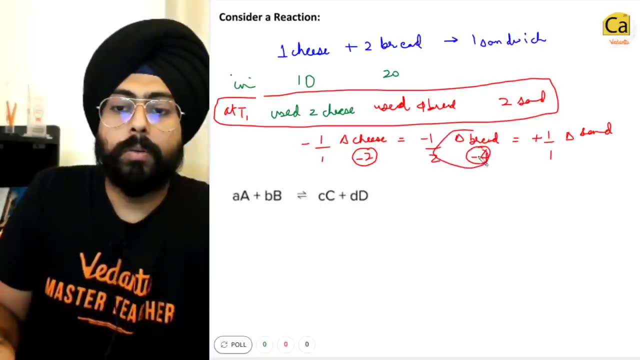 Since bread is decreasing, I will have to write minus 4.. Yeah, So since cheese is decreasing, delta cheese is minus 2.. Minus 2 into minus 1 is 2.. Minus 4 into minus 1 by 2 is 2.. 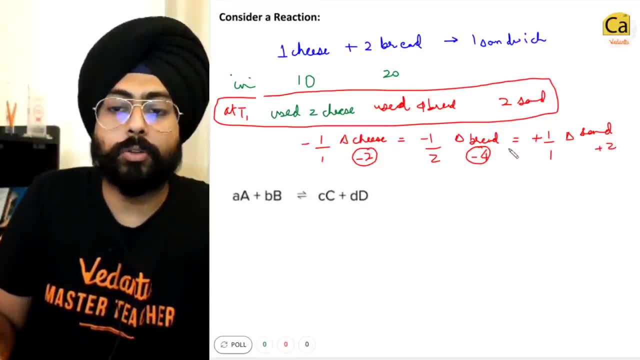 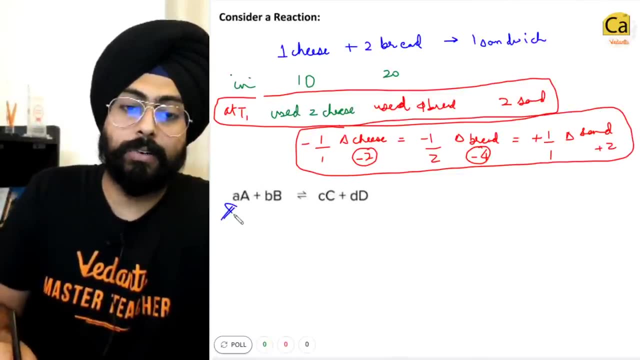 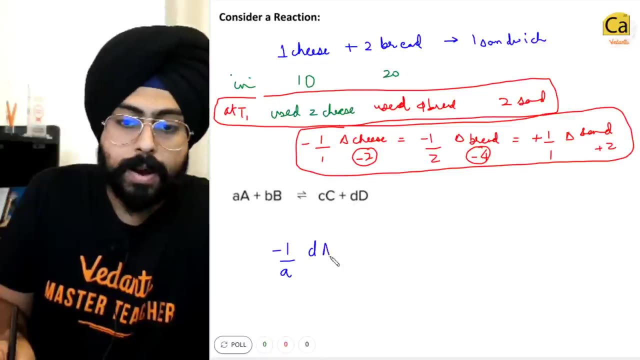 How many sandwiches are created? Plus 2.. Plus 2 into plus 1 is also equal to 2.. So I am pretty sure you understand this logic exists For a general reaction. now I will write it in a better handwriting. What you can write is: minus 1 by a, dA by dt. 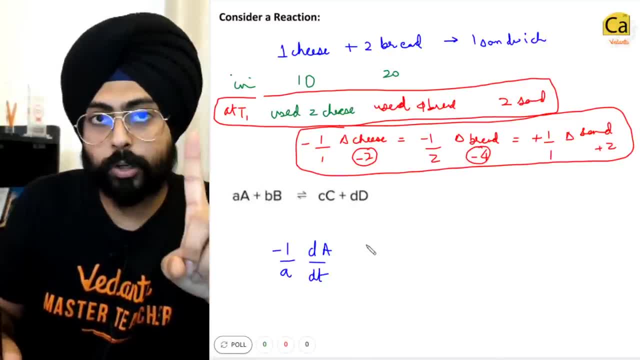 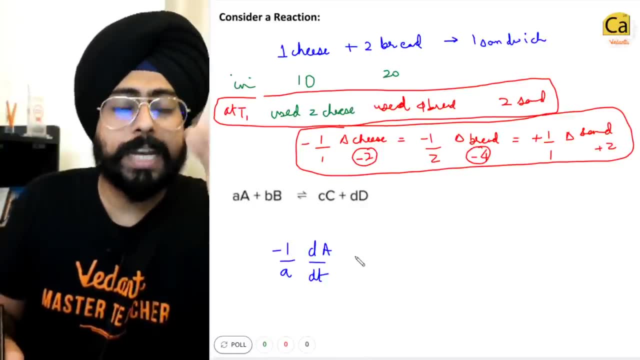 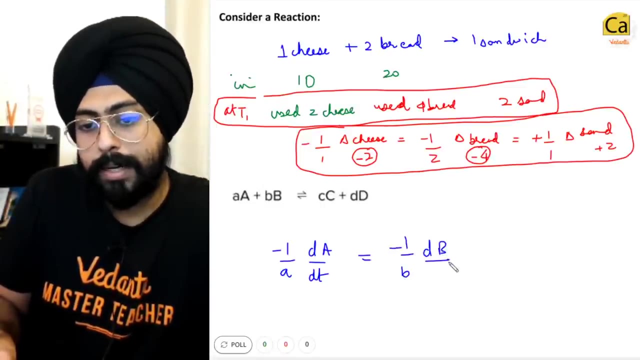 Okay, Where small a is the stoichiometric coefficient Capital, A is the change in the reactant. This could be the change in the concentration of reactants, change in the mole of reactants. Chalega, Okay, This is equal to minus 1 by b, dB by dt. 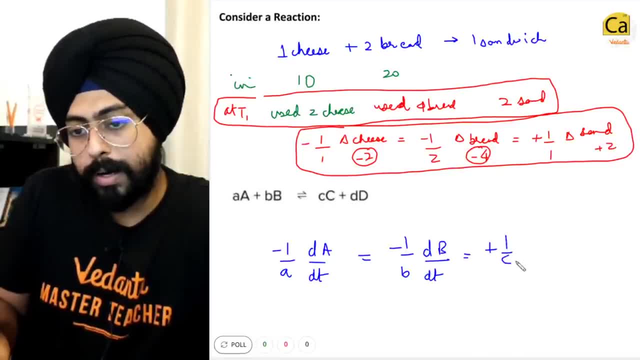 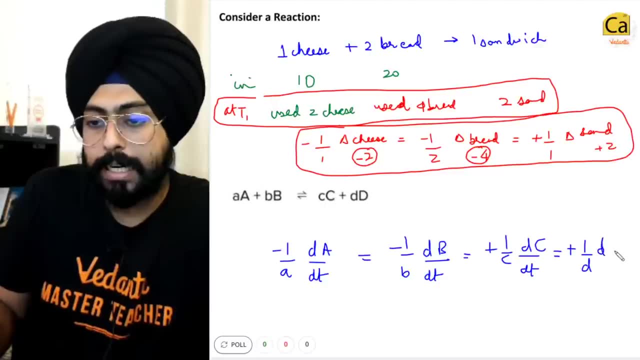 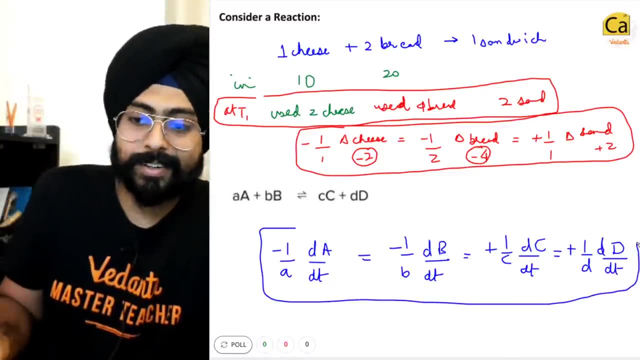 This is equal to plus 1 by c, dC by dt, which is equal to plus 1 by small d, d of capital, A, dT by dt. Right, I hope you remember this idea. Yes, I hope you remember this idea and I am pretty sure you have dealt with this idea in chemical. 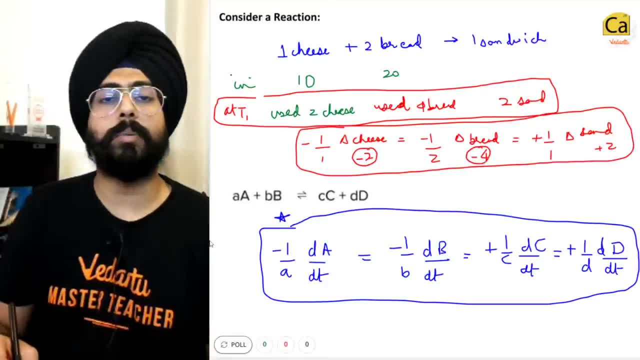 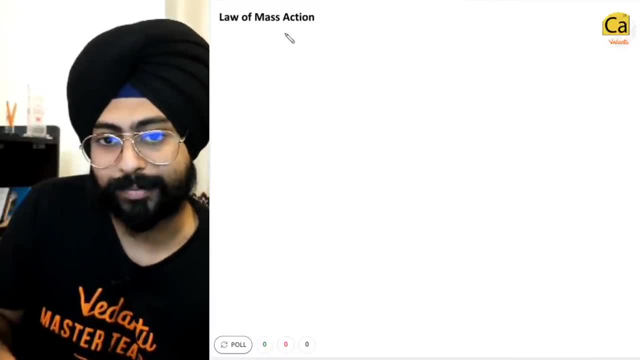 kinetics as well. Okay, So this is a very important idea for chemical equilibrium. Sometimes questions are asked according to this. Fine, Now let us move on into the law of mass action. What does law of mass action say? Law of mass action says that, let's say, you have a reaction like this: 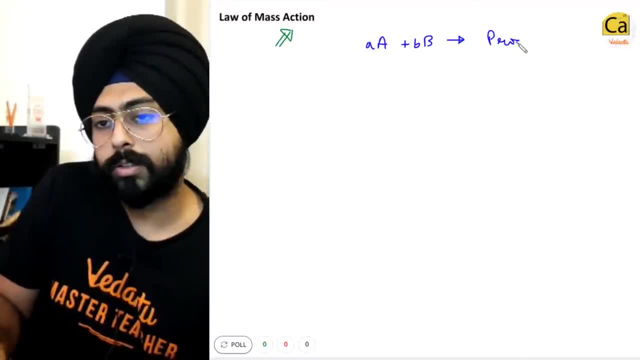 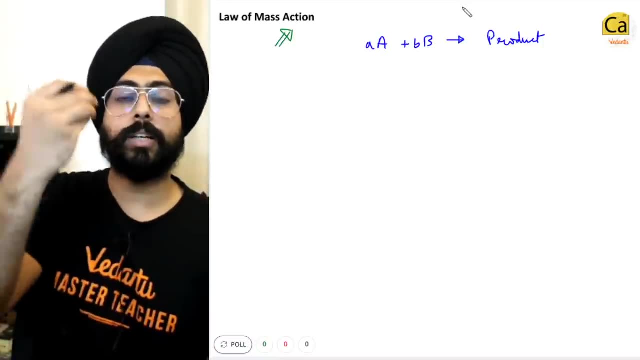 B times A plus B times B is going towards products. We don't care about what the products are. right now, Law of mass action is an empirical law. Empirical means it was determined experimentally sometime in the late 1800s. Okay, 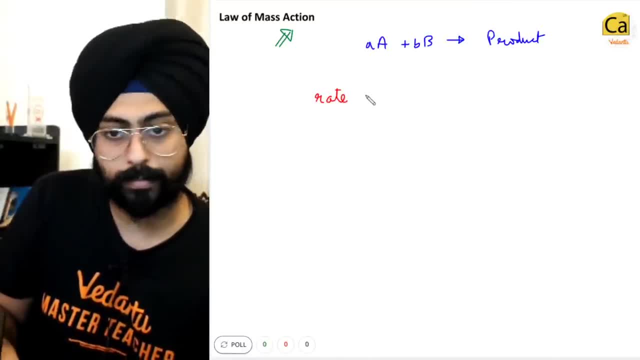 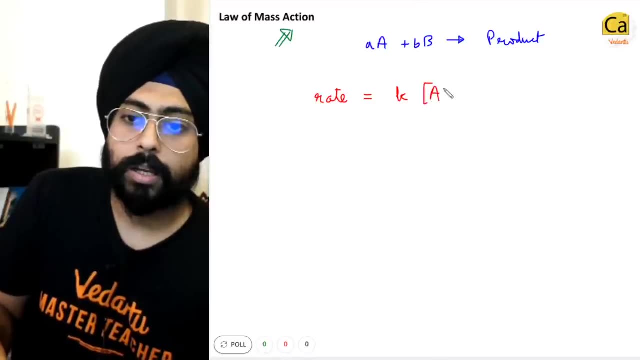 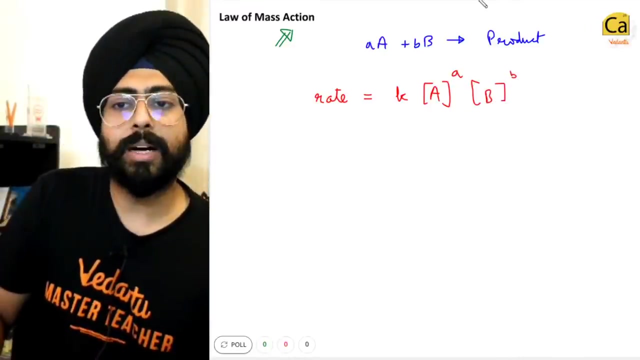 And this law essentially tells us that the rate of the reaction is equal to some constant K- Okay, Some constant K times active mass of A to the power A into active mass of B to the power B. What is this active mass? Active mass is essentially the part of the system participating in the reaction. 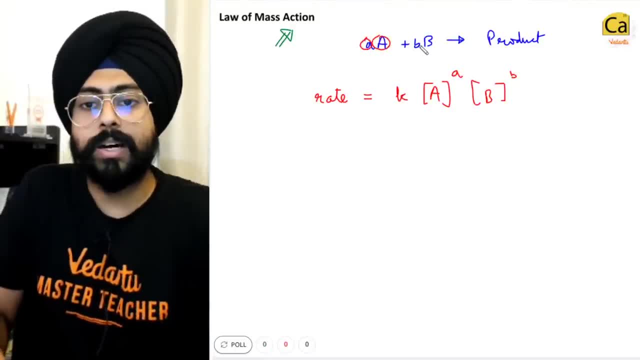 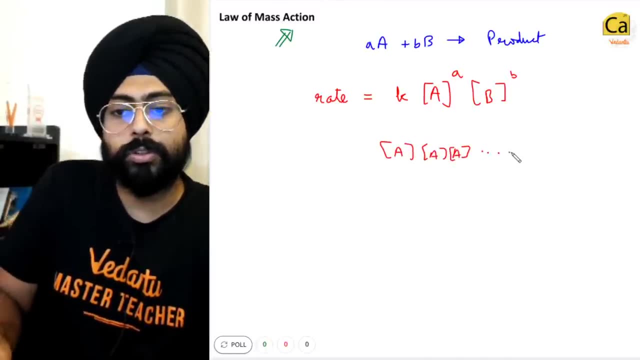 Okay, So over here what's happening is that A molecules of A are reacting with B molecules of B, So essentially you could write them as A into A, into A, so on and so forth, till you reach small a, B into B, into B into B, till you reach small b. 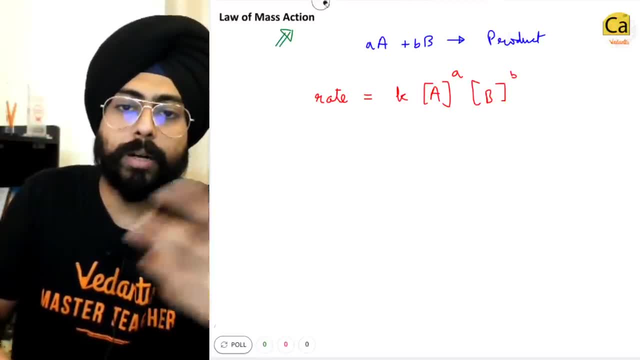 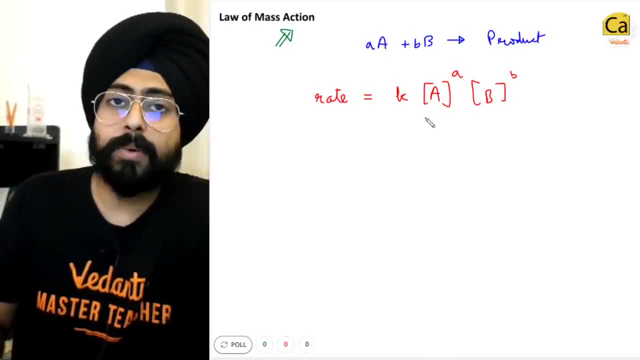 So, overall, this law can be written as: K into A to the power, A into B to the power B. So this is the law. Okay, Now these active masses could be concentrations, which is the most common way. These active masses could be partial pressures, which we will see in sometime. 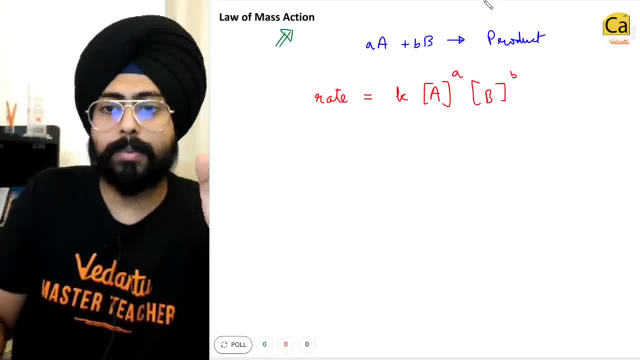 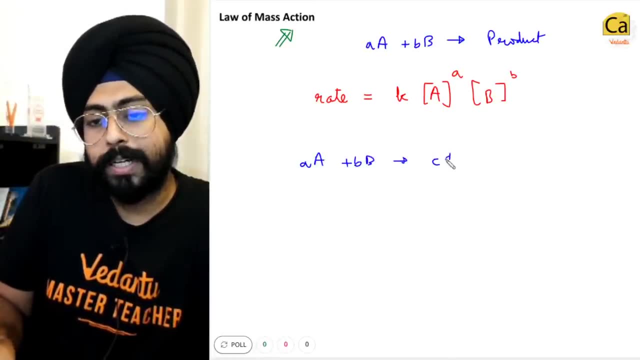 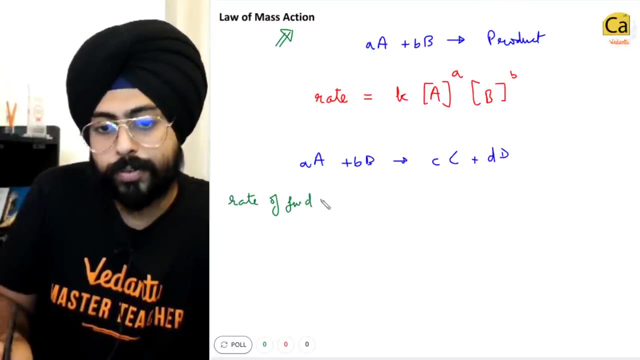 Yeah, So this is equal to rate. Everyone knows that. And, my dear friends, in case, okay, in case, you have A plus Bb, going to C times C plus D times D, can you write the rate of forward reaction and the rate of backward reaction? 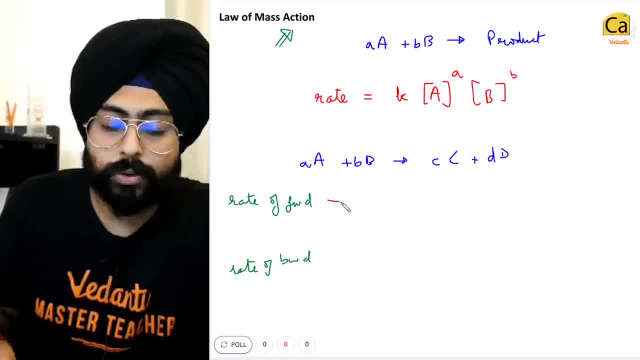 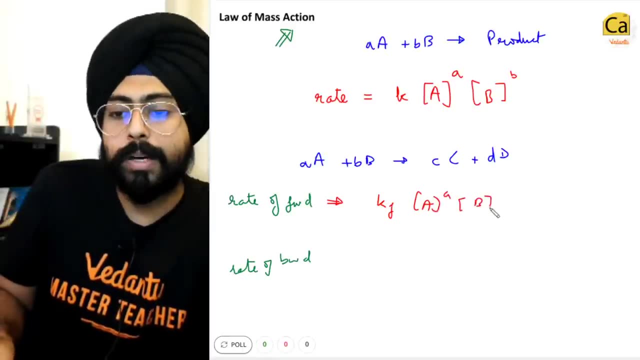 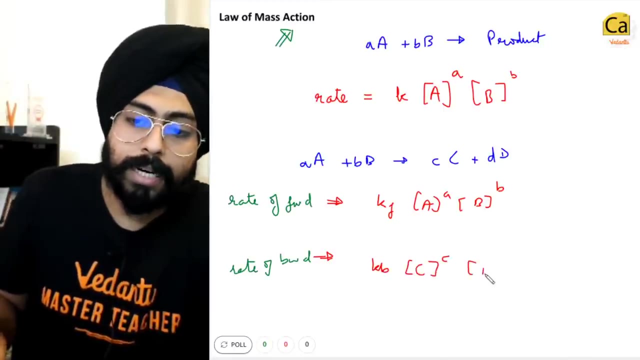 Okay, What is the rate of forward reaction? Rate of forward reaction is equal to K into. I will write Kf for K forward, A to the power A, B to the power B. K backward can be written as C to the power, C into, D to the power D. 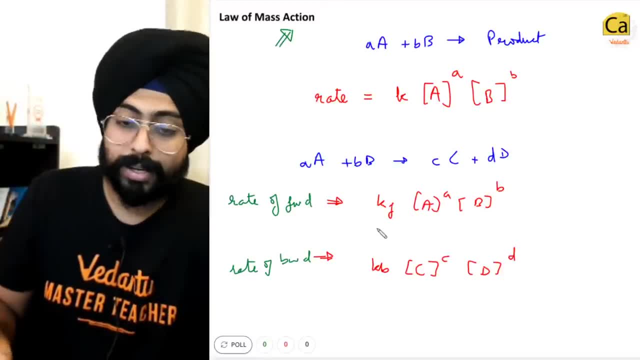 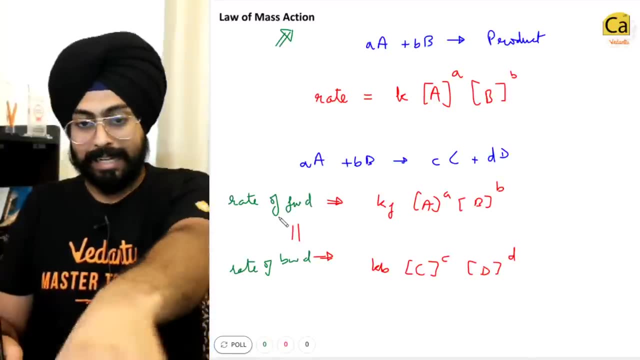 So, my dear friends, for the equilibrium, K forward is equal to K backward. sorry, rate of forward is equal to rate of backward. Yeah. So, my dear friends, Okay, Okay, In case you equilibrate these two ideas, okay, for equilibrium, constant Kc, what you will. 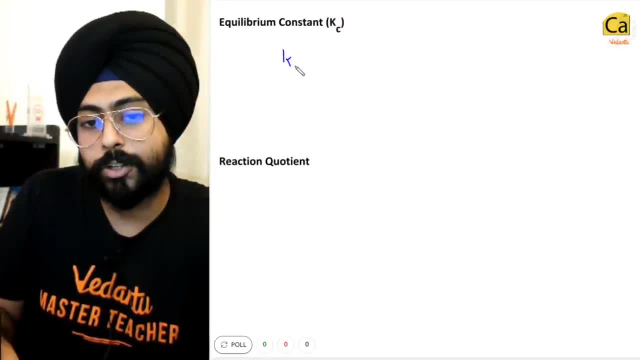 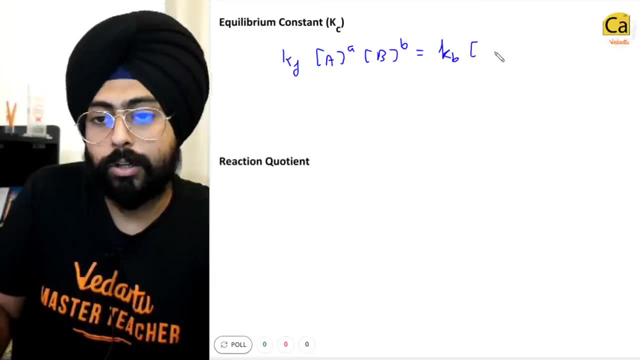 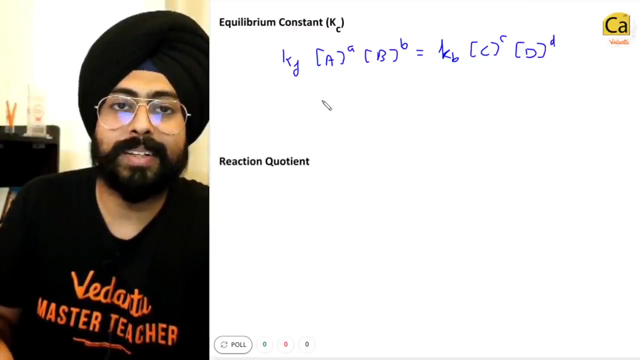 do is rate of forward reaction is equal to rate of backward reaction. So Kf into Aa, into Bb is equal to K backward, into Cc, into D, to the power D. So what does this give me, people? You get K forward by K backward is equal to the equilibrium constant Kc. 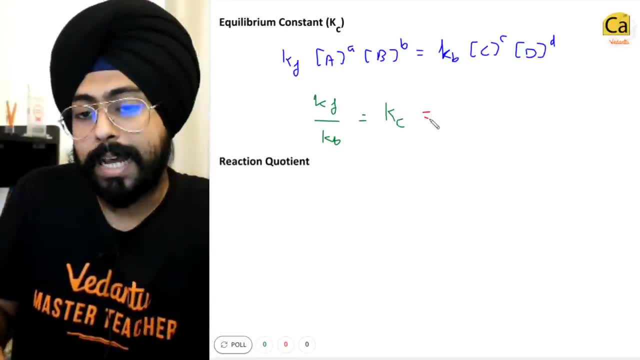 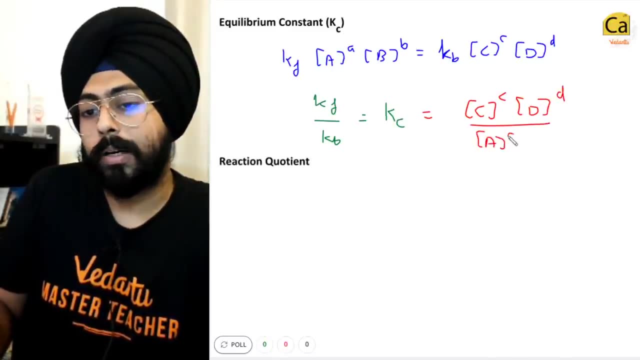 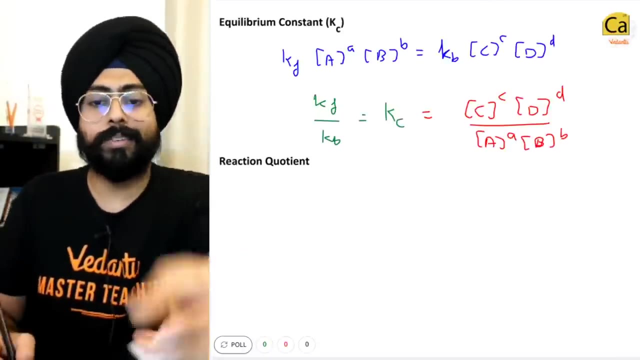 C means Equilibrium, constant in terms of concentration, and this is equal to C to the power C, D to the power D upon A to the power A into B to the power B. Very simple, very obvious. yeah, So simple that we were able to derive this idea in the revision class itself. 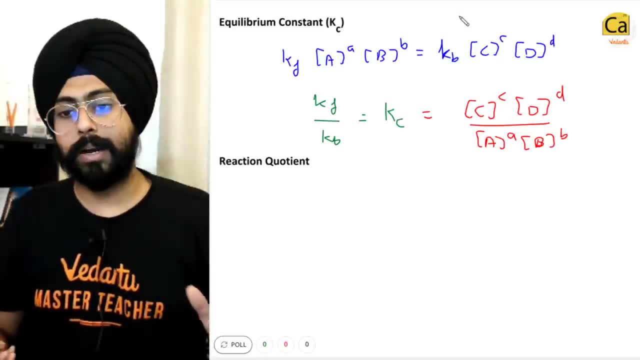 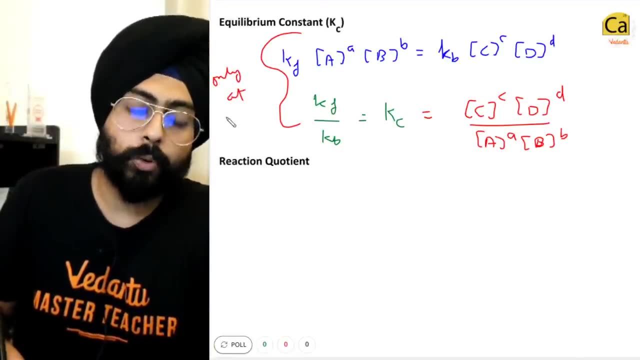 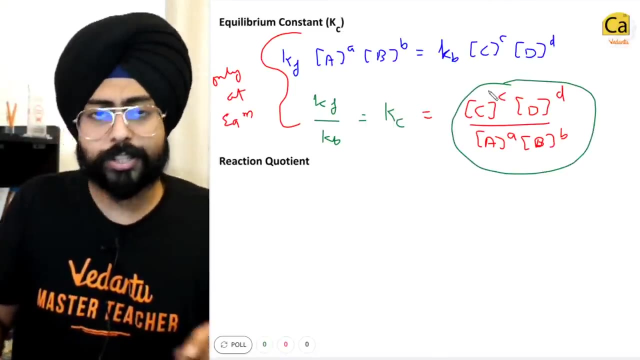 Equilibrium: constant Kc, which is equal to K forward by K backward, which is this. Now, my dear friends, do you realize that this condition is applicable? Okay, Only at the equilibrium. This condition is applicable only at the equilibrium, But you could do this calculation outside of the equilibrium as well, right? 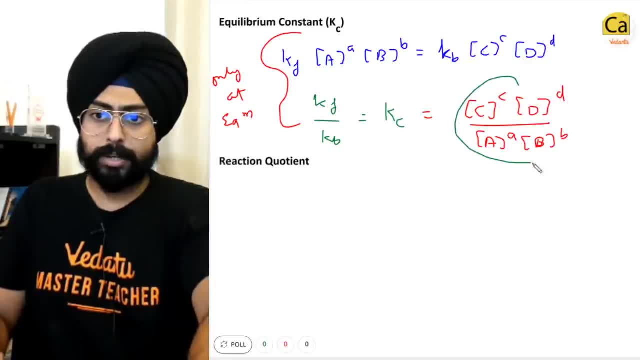 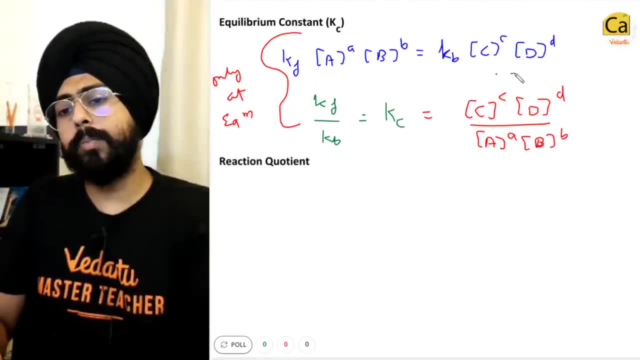 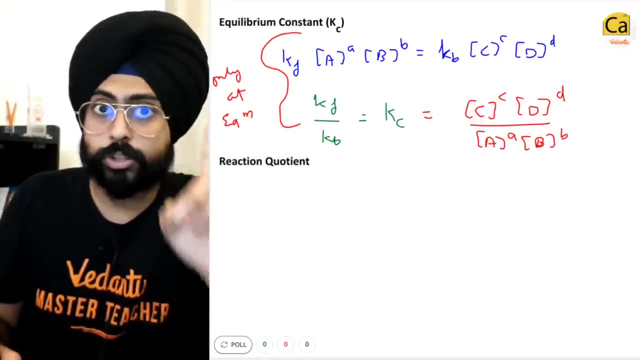 In the chemical laboratory, when you start a reaction, you can make the measurements of concentrations and come up with this: The thing that I am circling in black. Only at equilibrium is this black circled thing equal to Kc, Sir for sir of equilibrium. 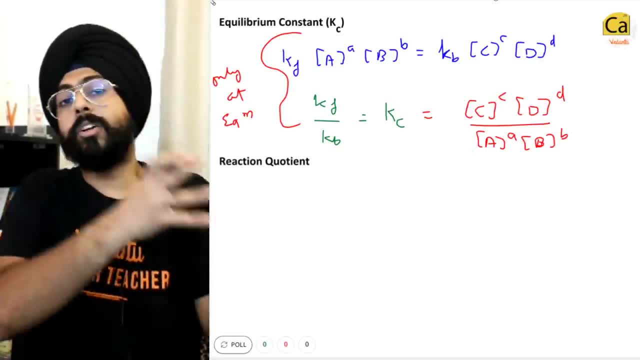 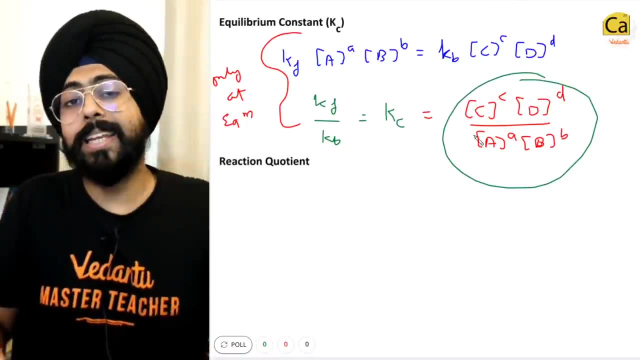 At equilibrium. this will be called equilibrium constant. At other concentrations, apart from the equilibrium, let's say you just started the reaction and measured the concentrations. Then, my dear friends, in any other general condition, this black thing is known as the reaction quotient. okay, 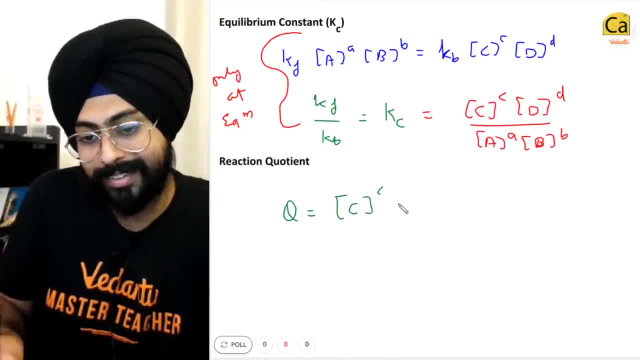 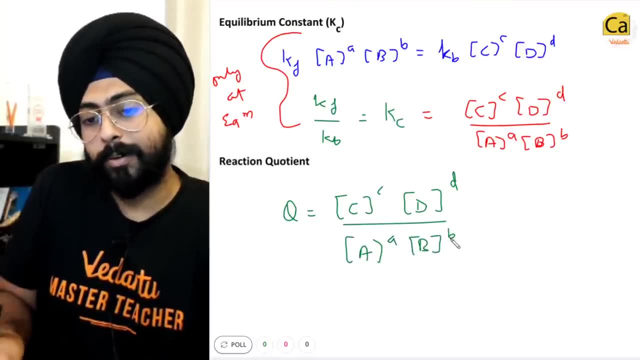 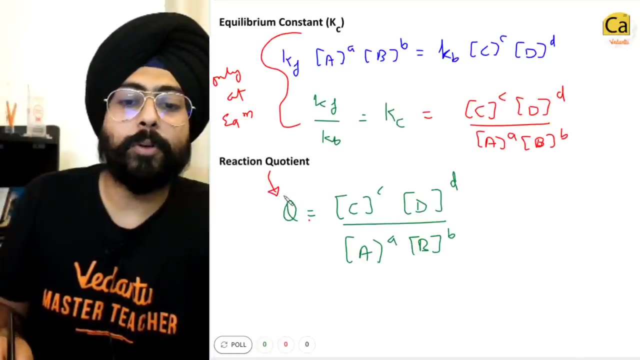 So reaction quotient is also the same thing. I will write it. Writing this is the toughest thing about this. chapter B to the power B, okay, And this is known as the reaction quotient, And these are applicable at any point of time other than the equilibrium. 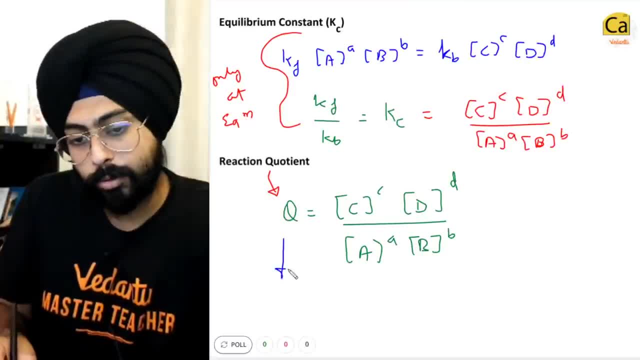 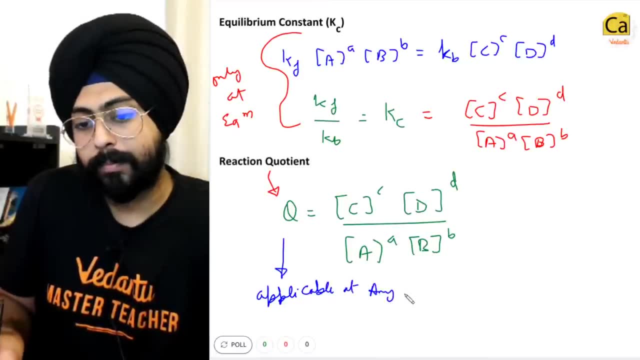 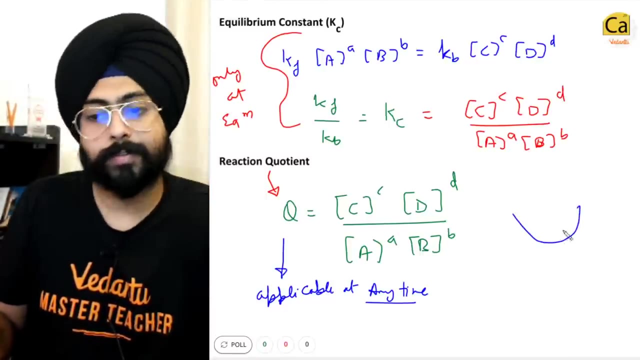 Okay, So here I will write this idea in blue color as well, that this is applicable at any point of time, Not just the equilibrium, okay, So now, my dear friends, do you remember I told you about this system of the ball? okay. 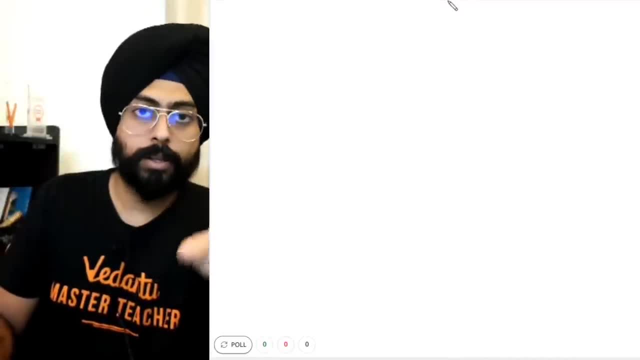 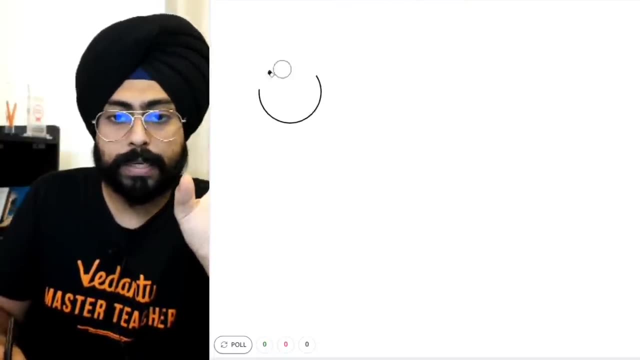 Let's try to write down the relationship between reaction quotient and reaction quotient. Let's try to write down the relationship between reaction quotient and reaction quotient And k-equilibrium- What you need to do in order for yourself to remember- okay, Some people get confused in this idea. 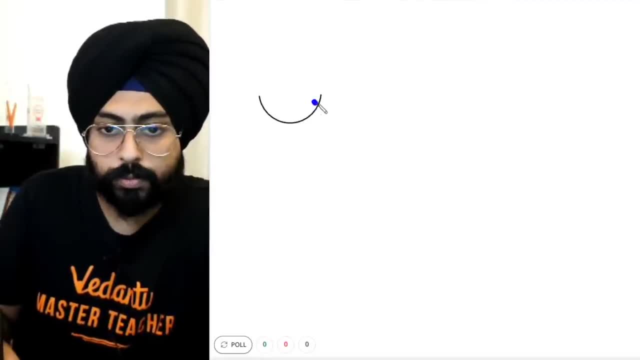 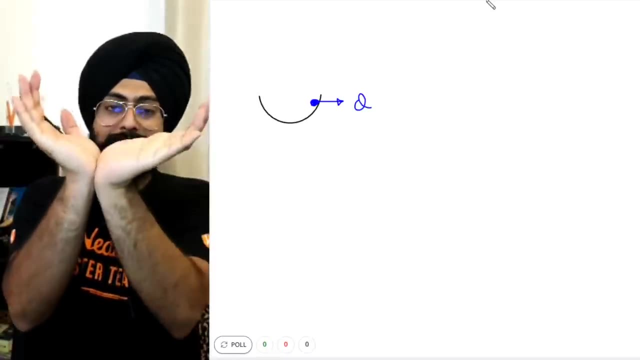 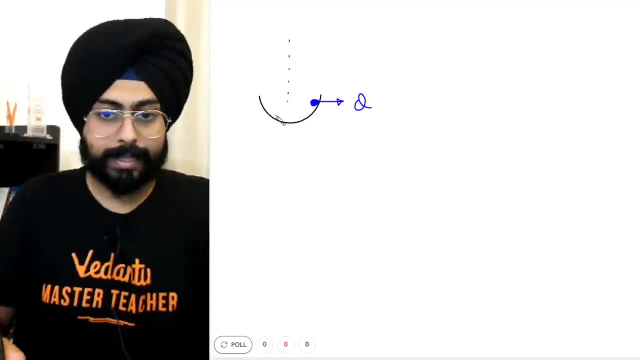 I will tell you how to remember. okay, Think of this ball. okay, Think of this ball as the reaction quotient and think of this entire thing as the reaction. This entire system is the reaction. okay, Now, my dear friends, this middle line that we have, okay, this middle point that we have, 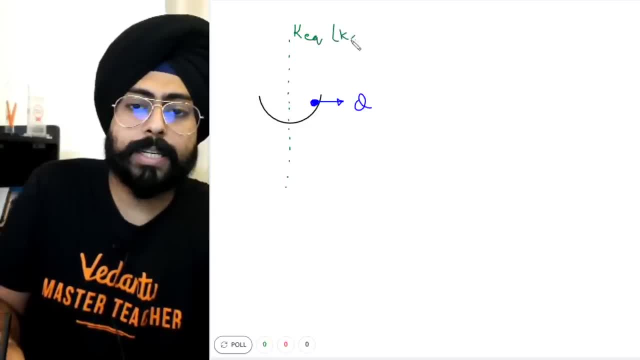 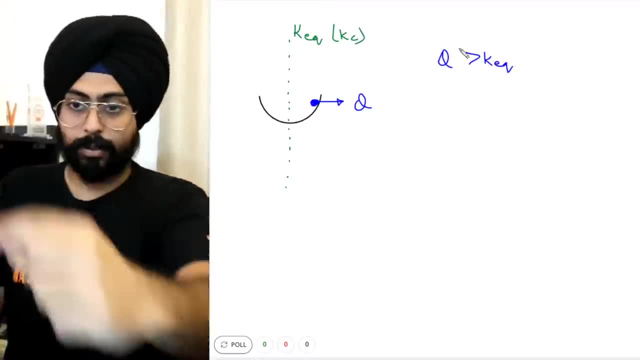 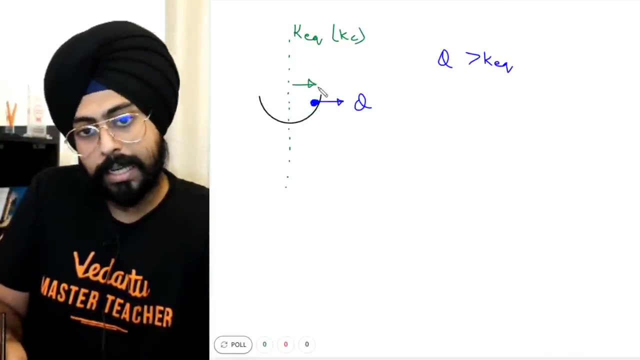 this is the point of K equilibrium. let's say Kc. Now, my dear friends, if Q is greater than K equilibrium, if Q is greater than K equilibrium, which is the example that we have given over here, the ball will move back. if my Q is ahead of the K equilibrium, my 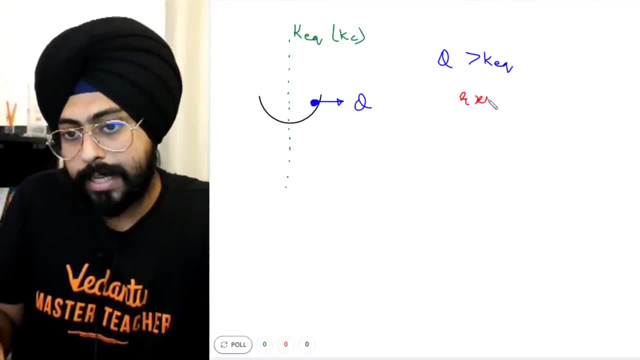 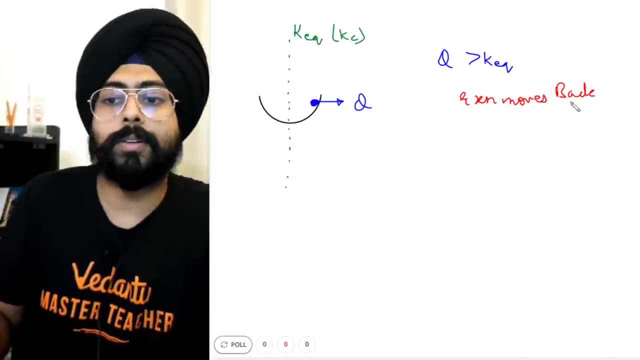 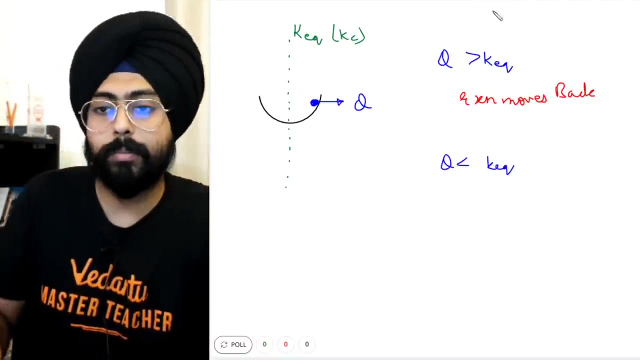 ball will move back. so in this case, the reaction moves backwards. realize this: Q greater than K equilibrium. reaction moves back. similarly, Q less than K equilibrium. just imagine this system in your brain: Q is less than K equilibrium. it will move forward. as simple as that it. 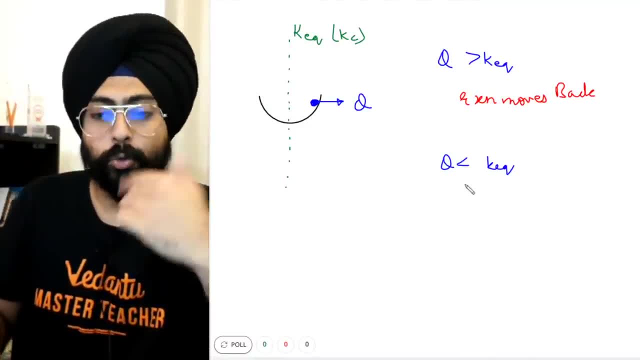 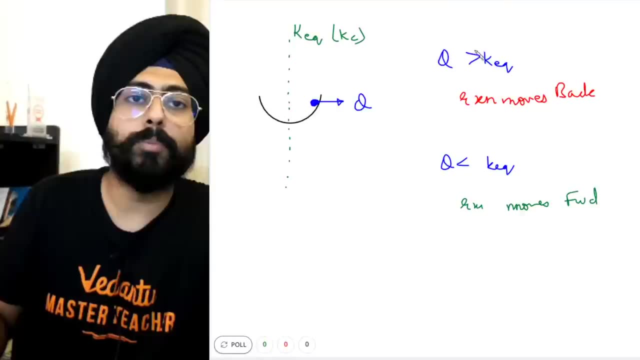 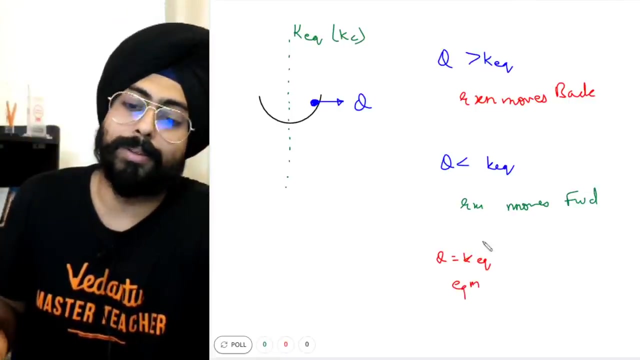 will move forward. yeah, this imagination helps now. So Q less than K- equilibrium Reaction moves forward. as simple as that. alright. and finally, if Q is equal to K equilibrium, then we call it the equilibrium. as simple as that, okay. 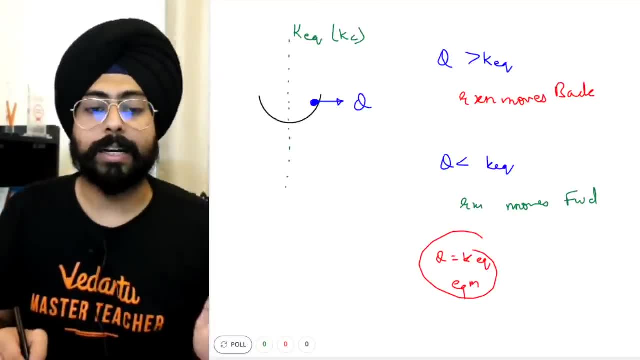 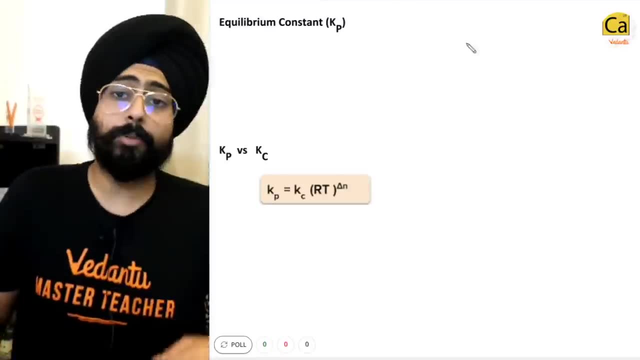 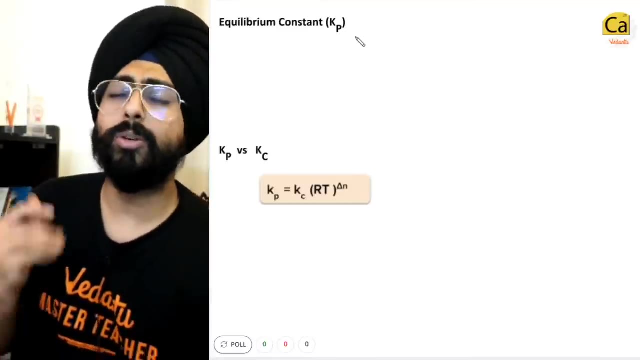 So equilibrium constant, reaction quotient, equilibrium is attained. the system always wants to attain equilibrium, very, very simple. Now, my dear friends, there is another equilibrium constant called the equilibrium constant, called Kp, and this is generally used for gaseous reactions. you can also use it for 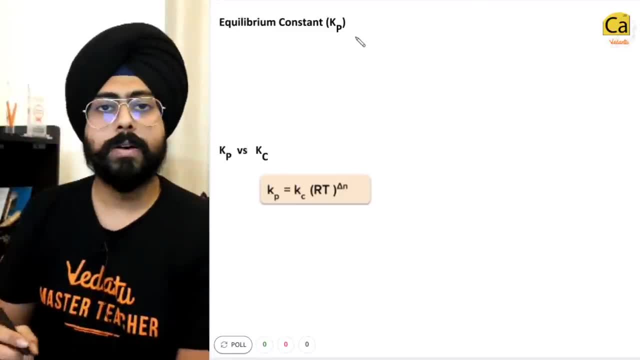 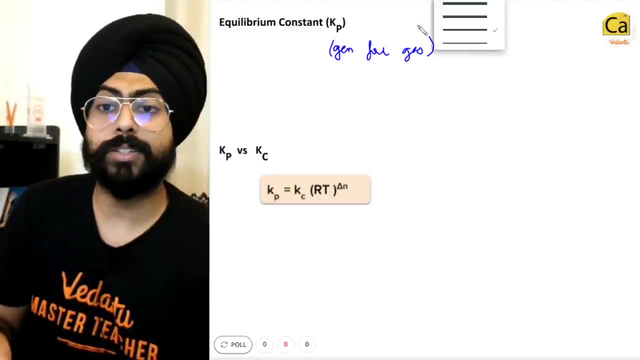 liquid reactions where there are partial pressures. okay, So generally for gaseous reactions. so let's say you have a gaseous reaction, you have H2 plus N2 giving you NH3, likh sakta hu main. fine, this is the reaction that I can write. 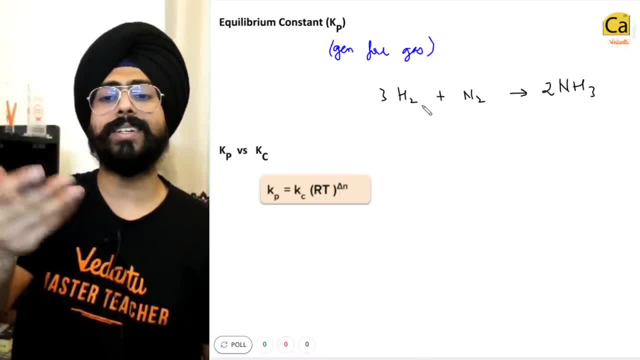 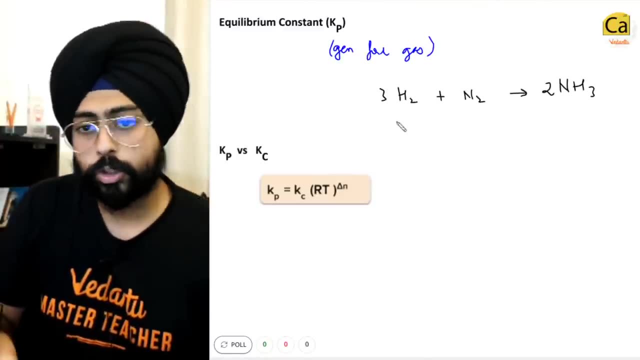 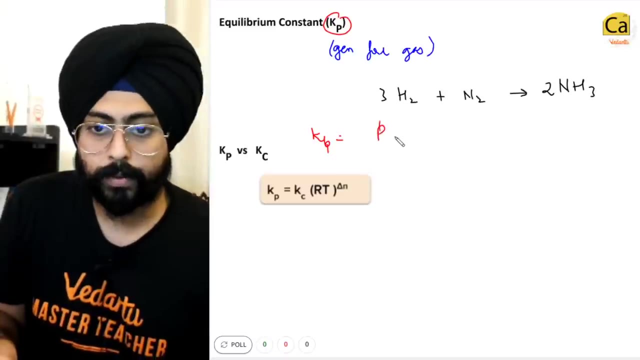 so, over here, do you realize that instead of talking about concentrations, it's easier to talk about partial pressures of these gases? because H2, N2 and ammonia, all of them, are gases. okay, So since these are gases, I can write Kp to be equal to the partial pressure. okay, the? 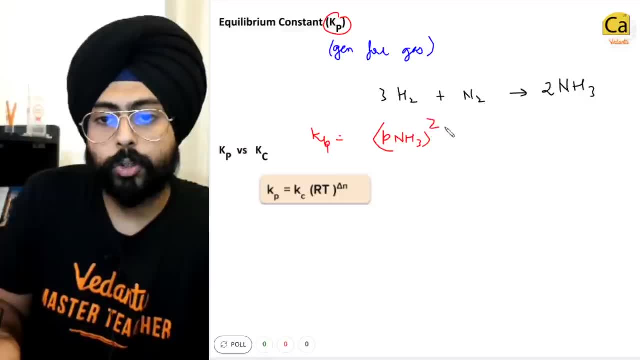 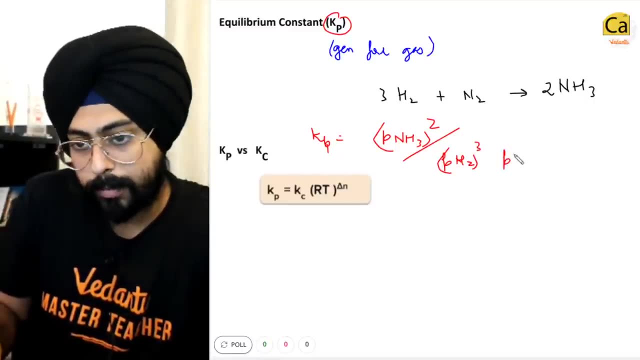 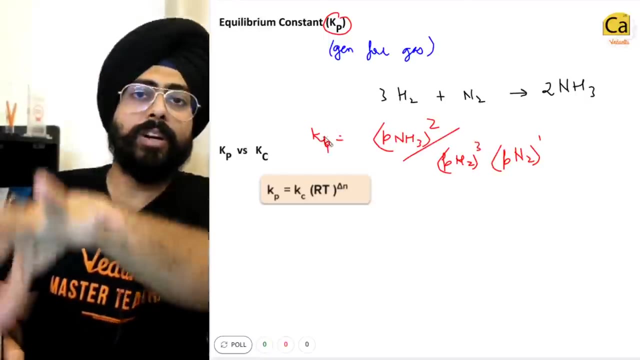 partial pressure of NH3 raised to the power 2 upon the partial pressure of hydrogen raised to the power 3.. Okay, So partial pressure of nitrogen raised to the power 1.. This is known as Kp. it's just a different way of writing the equilibrium constant talking. 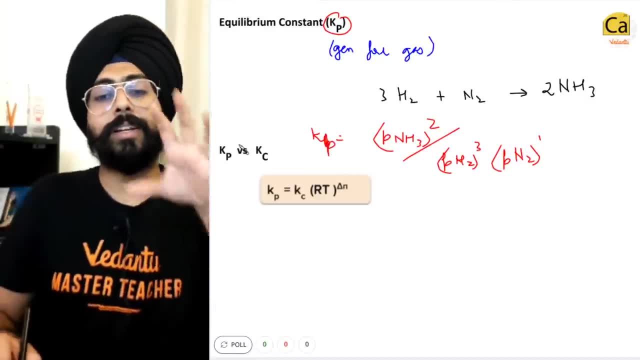 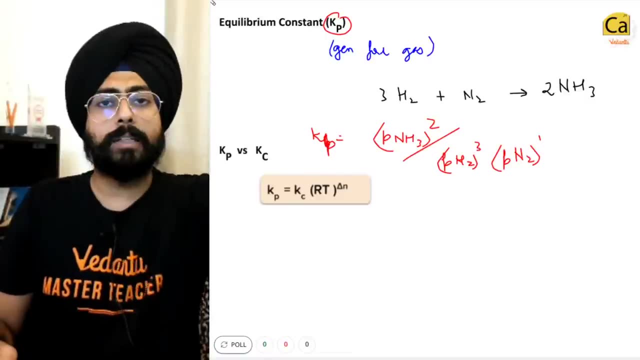 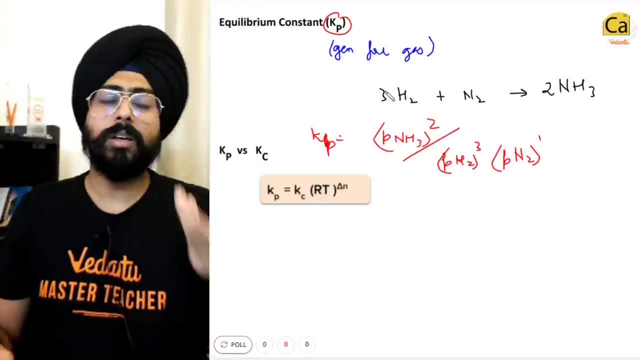 about partial pressures rather than concentrations. If there is a system in which you can have both Kp and Kc, for example over here, you could write concentration as well, isn't it? moles per liter that is concentration. so moles of hydrogen per volume of this entire mixture, it can give you a concentration of 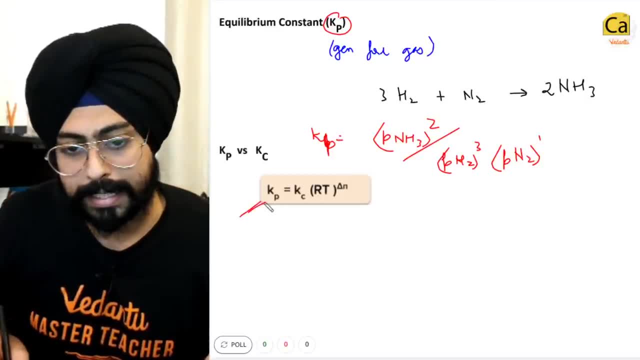 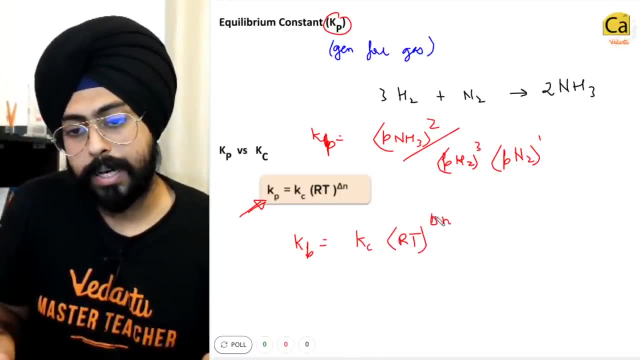 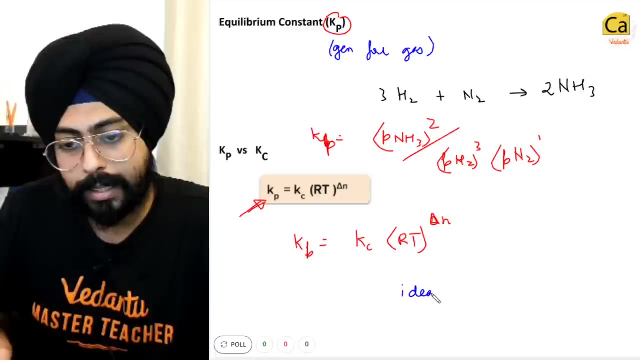 hydrogen. So the relationship between Kp and Kc is this: Kp is equal to Kc into RT, to the power delta N. What are our assumptions over here? The assumptions over here are that we are assuming ideal gas behavior. okay, this is. 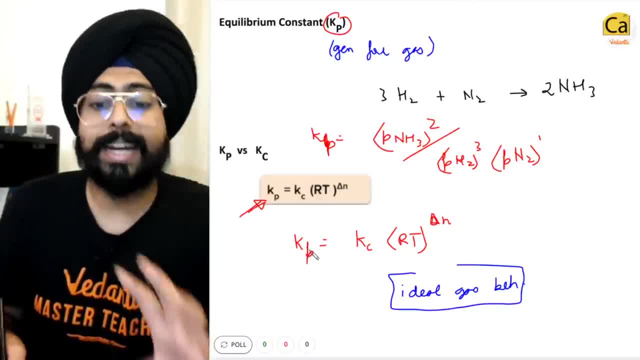 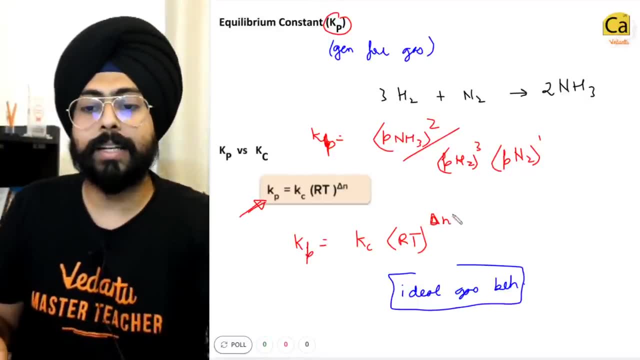 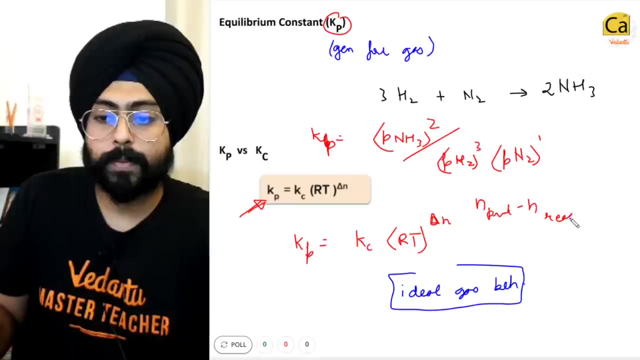 an implicit assumption whenever we convert Kp into Kc that we are following an ideal gas behavior. okay, okay, Okay. So what is delta N? Delta N is the number of moles of products minus number of mole of reactants. fine, 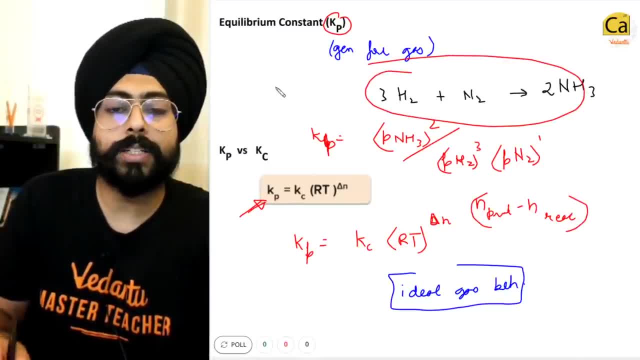 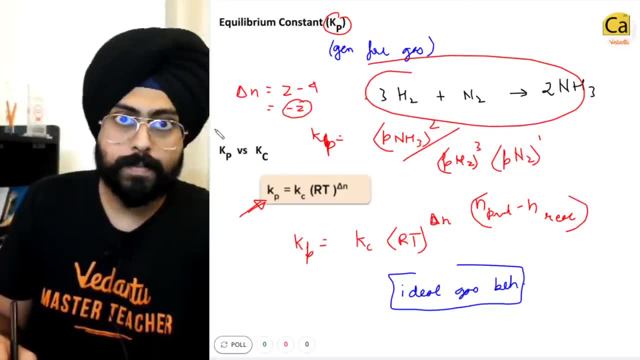 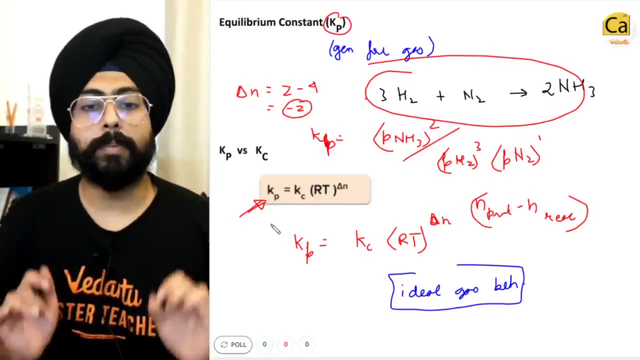 So over here, can you tell me what is delta N in this particular reaction? what is delta N? Delta N is equal to 2 minus 3 plus 1, that is 4, that is equal to minus 2, total number of moles of gas are decreasing in this reaction, so this is the idea that will be applicable. 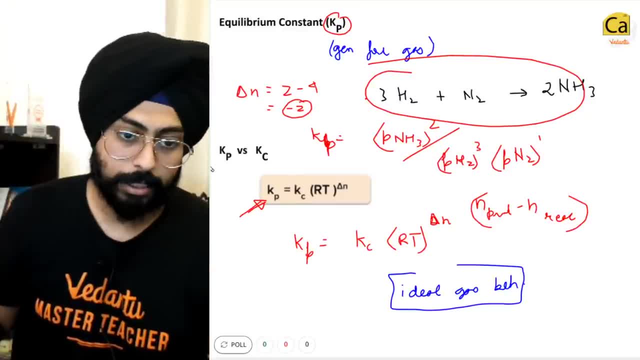 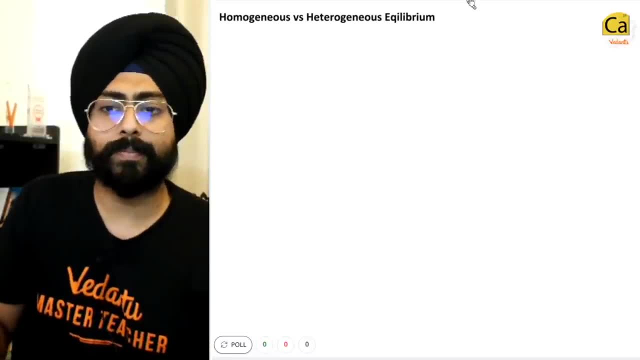 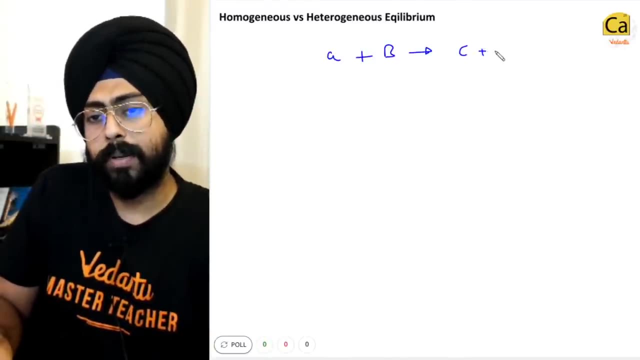 Kp is equal to Kc into RT, to the power delta N. Now let us talk about homogenous versus heterogeneous equilibrium. homogenous equilibrium is simple. homogenous equilibrium is A plus B, going to C plus D, and all of these are, let's say, liquids. 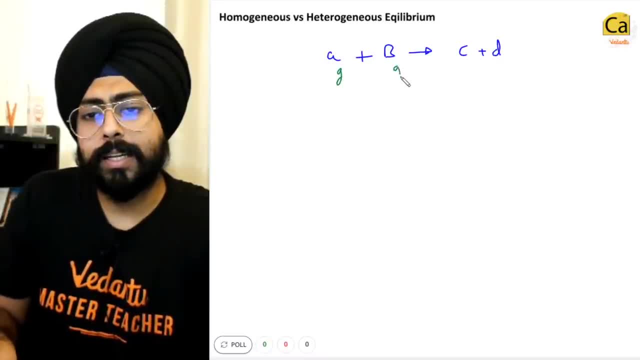 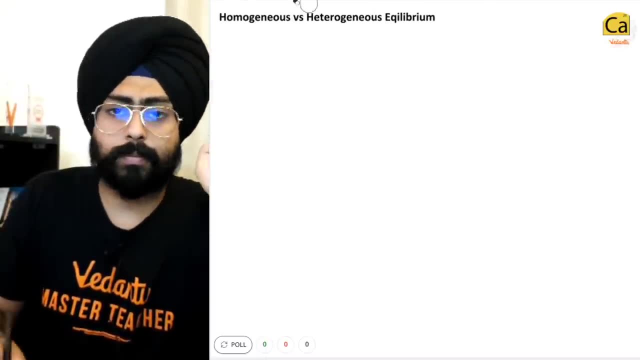 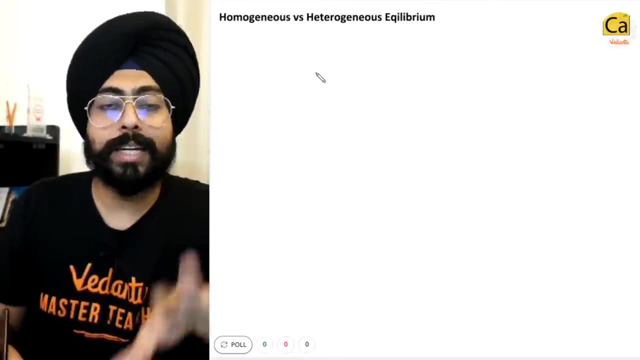 all of these are, let's say, aqueous. all of these are, let's say, gases. this is a homogenous equilibrium. It is very simple to write the law. it is very simple to write the K equilibrium. but heterogenous equilibrium may you can have solids and liquids and gases, all of them. 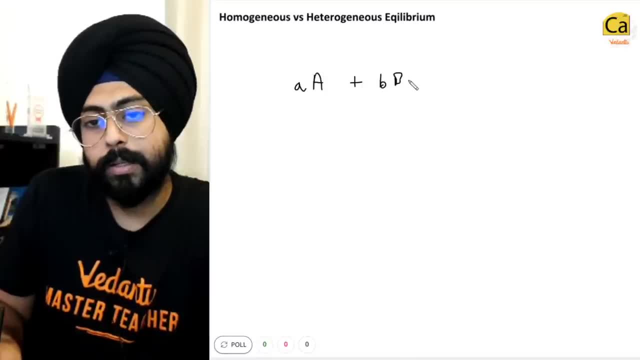 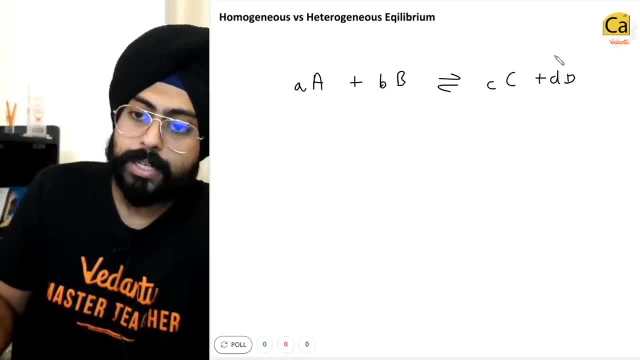 So your reaction will look something like this: where A plus B is going towards, let's make an equilibrium reaction- C times C plus D times D, and let's say over here: A is a solid, B is gaseous, C is gaseous, D is gaseous. 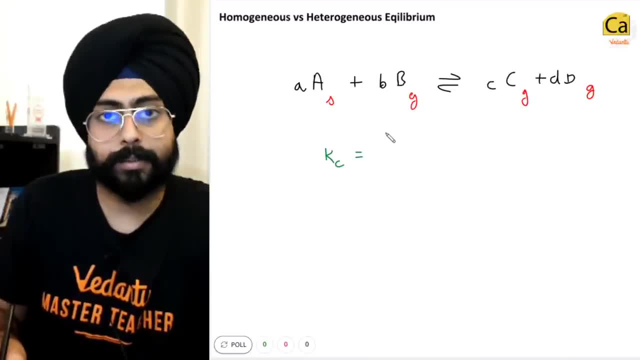 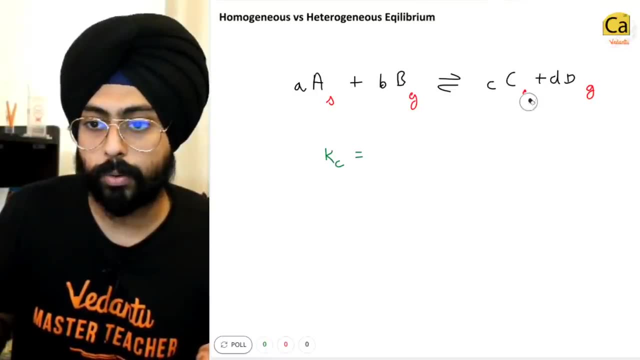 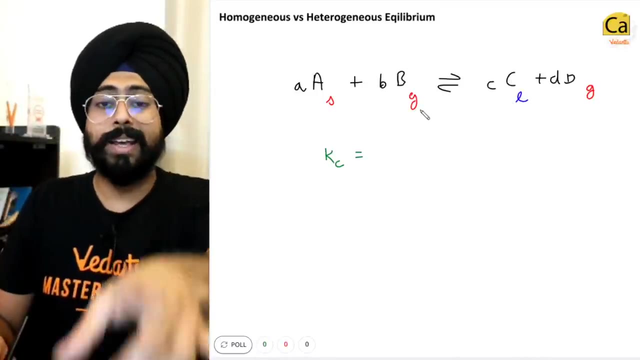 So in this particular case, the Kc that you will write okay, includes only the most volatile phase. okay. in case C was a liquid over here, okay, this is a very rare case, no one is going to ask you this. but in case C was a liquid, A is a solid, then you will include. 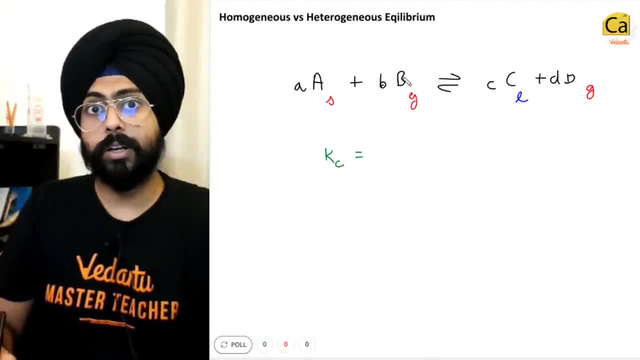 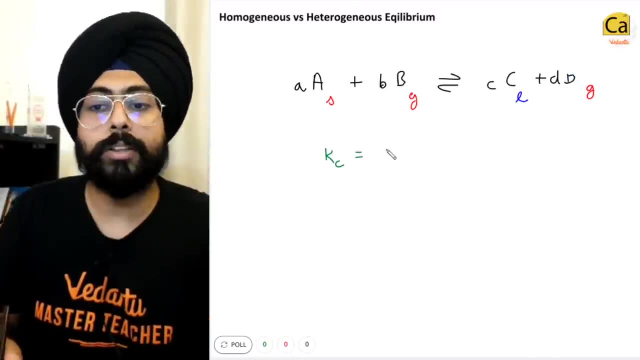 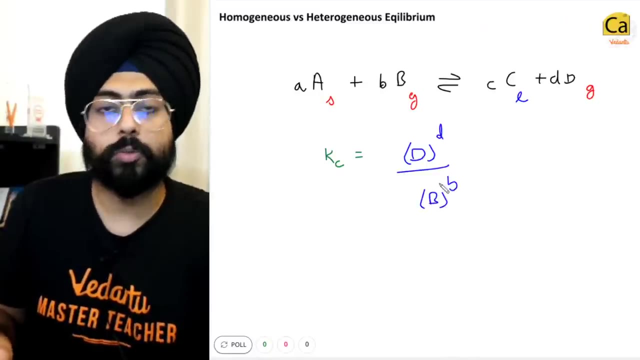 only the most volatile phases. what is the most volatile phase over here? what is the most random phase over here? gaseous phase. so the equilibrium constant will be written only in the terms of gaseous. okay, D to the power, D upon B to the power, small b if. 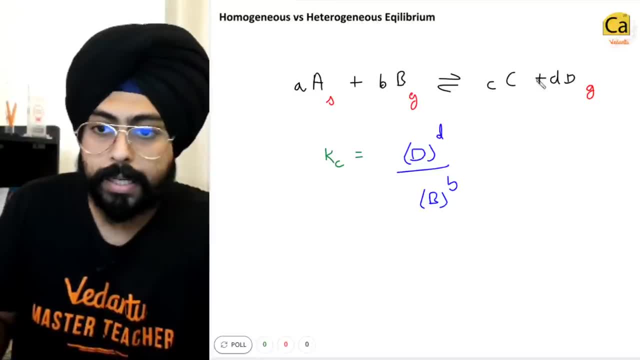 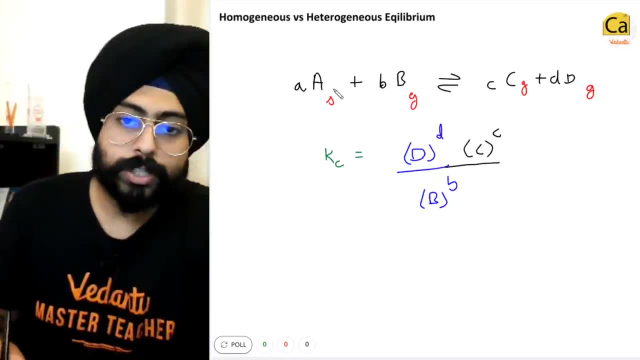 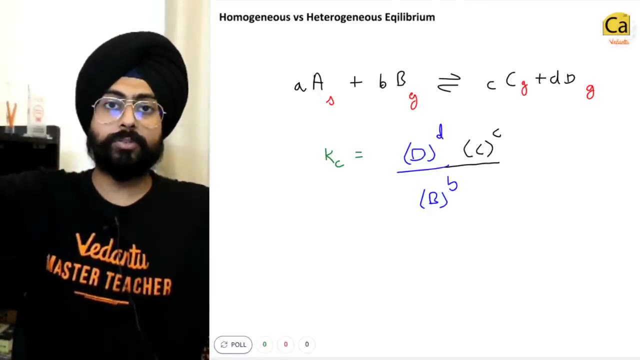 C over here was gaseous. yeah, then you will include that into your rate law as well. as simple as that. so you just have to ignore the less volatile phases because, think about it, solid gas, gas now, all the difference that is happening inside the volume of the 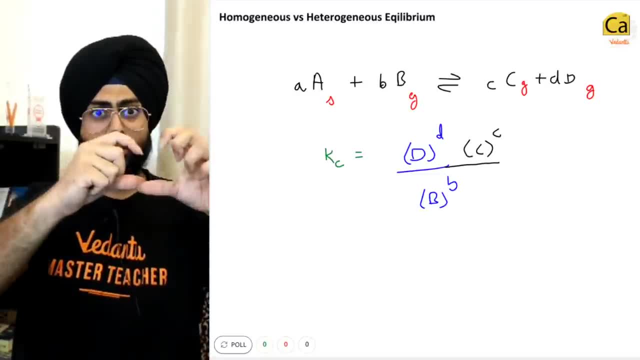 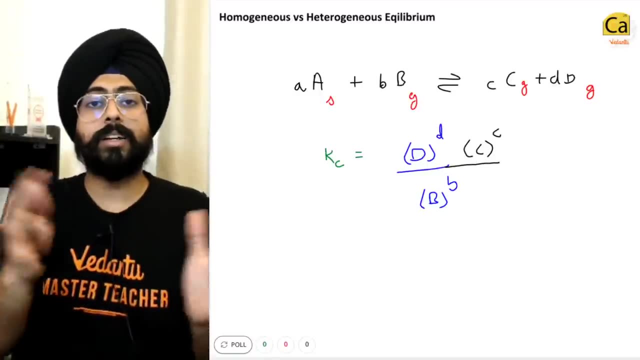 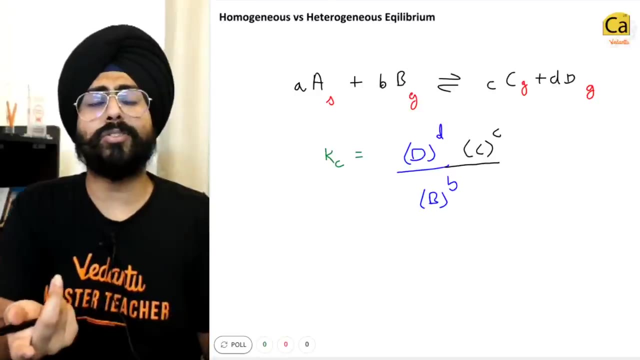 reaction mixture will be because of the gas right Solid. Solid volume will hardly change compared to the gaseous volume. so the mass action that is happening, the active masses that are changing, will be a lot more drastic for gases. concentration of the gases will change a lot. concentration of the solid: negligible. 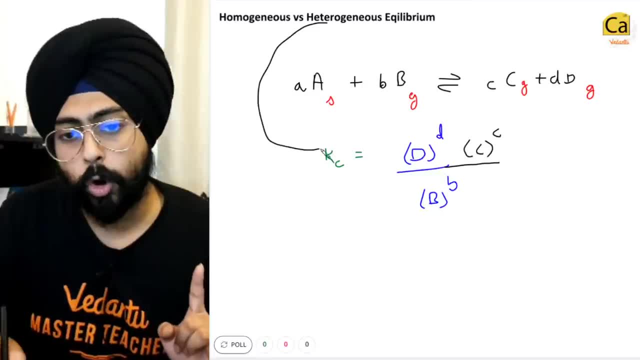 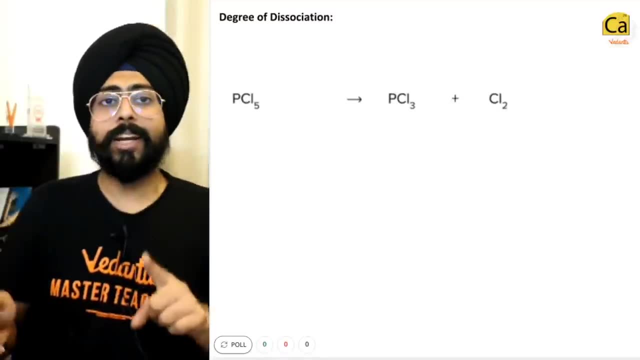 compared to the gases. fine. so in heterogeneous equilibrium, only take the most volatile phase. very nice, very simple thing. let's move on then. do you remember what is degree of dissociation? Degree of dissociation is Alpha. how do we do the calculation? 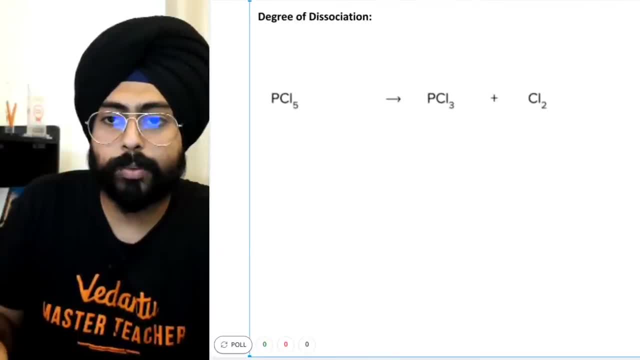 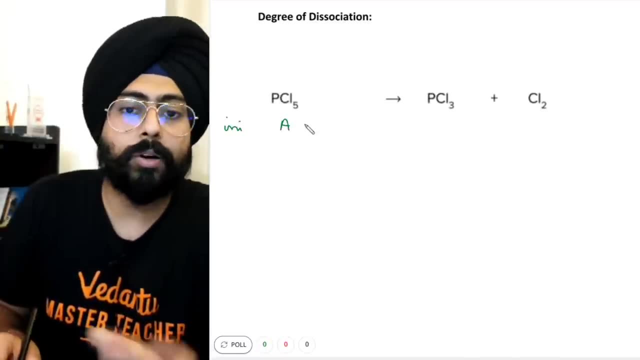 I have taken a reaction over here for you guys, for me to be able to explain it. how will we do this? PCL5, let's say, initially, you have capital, A amount of this, 0 of this, 0 of this at. 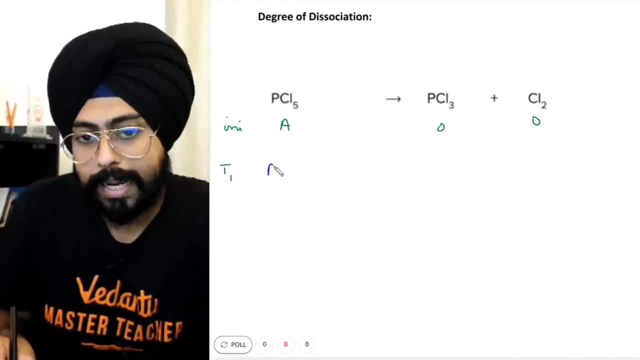 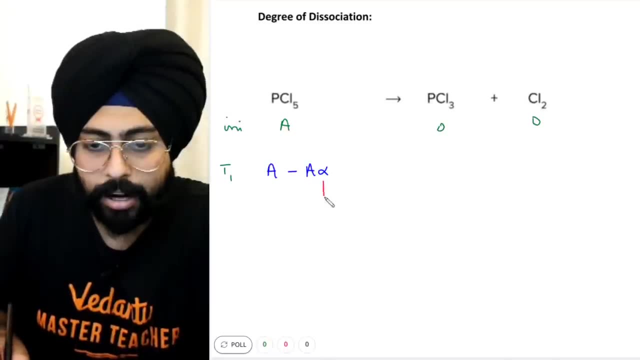 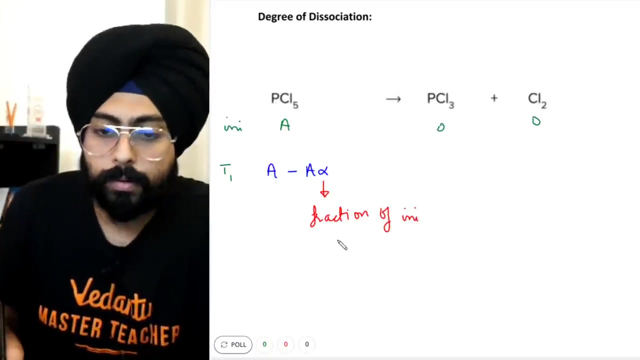 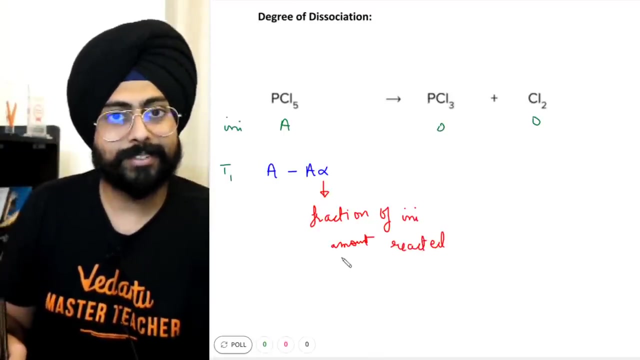 time T1,. what we can write is A minus A alpha is reducing. what is this alpha now? This alpha is basically the fraction Of the initial amount. okay, this is the fraction of the initial amount that has already reacted. fine, this alpha is the fraction of the initial amount that has reacted. let's 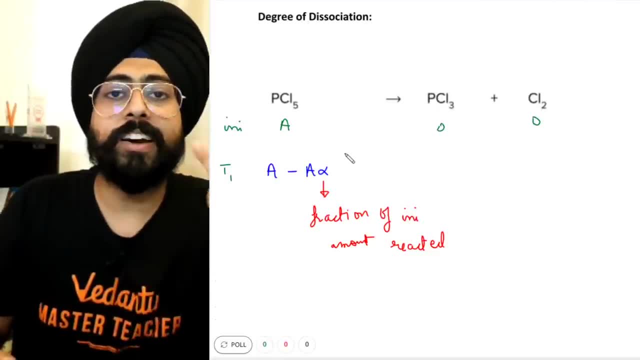 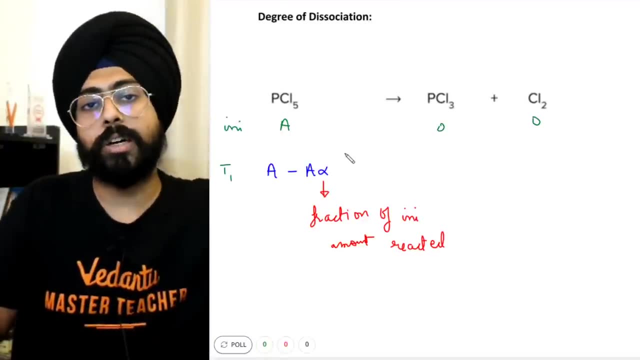 say. I say you had 20 apples, I took away 5% of the apples, something like that. okay, to take a very easy example, let's say you have 100 apples, I take away 5% of apples. 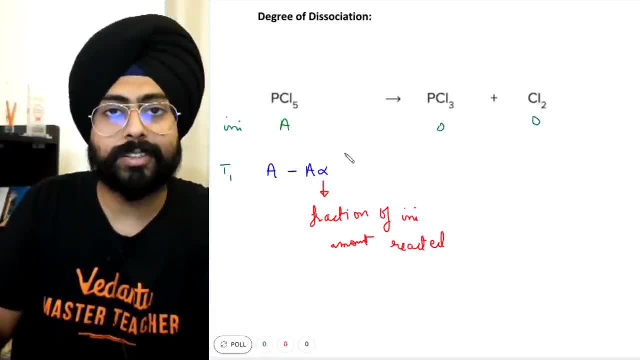 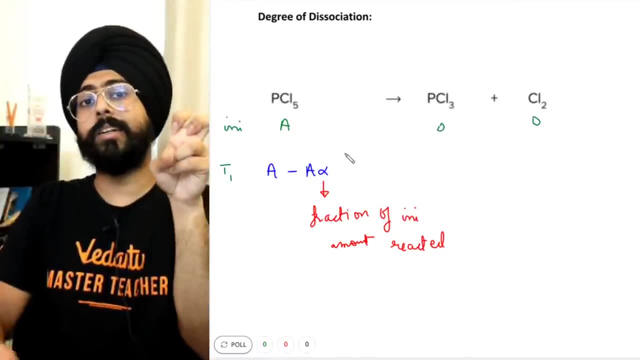 how many apples do you have? now You can do the calculation: Yeah, You have 100 minus 5, 95 apples. very simple, yeah, So that 5% is exactly what is alpha, the fraction or the percentage of the initial. 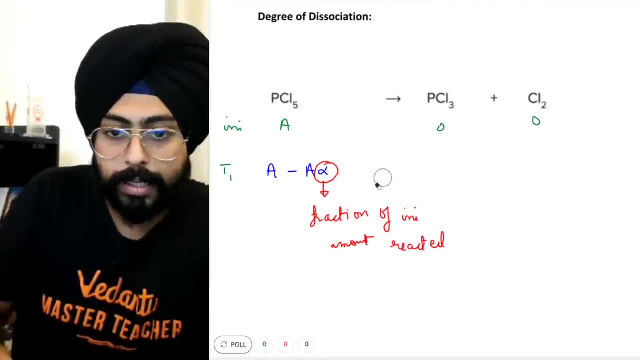 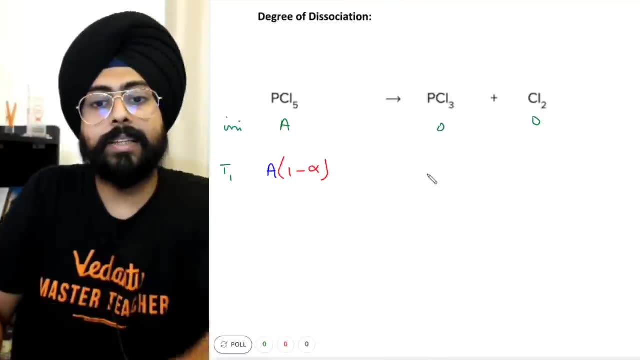 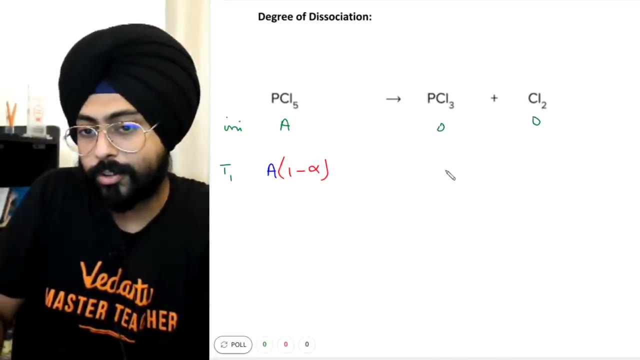 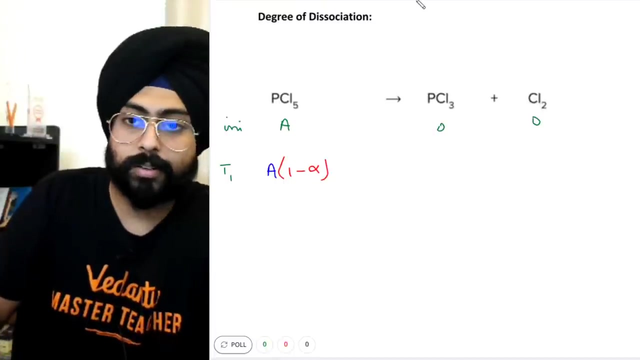 amount taken away. okay, So here I can write it as A into 1 minus alpha. PCL3 will simply become: how much will it become? Reduction over? here is A alpha, so this also becomes A alpha. this also becomes A alpha. is that fine? okay, got it alright, alright, nothing. 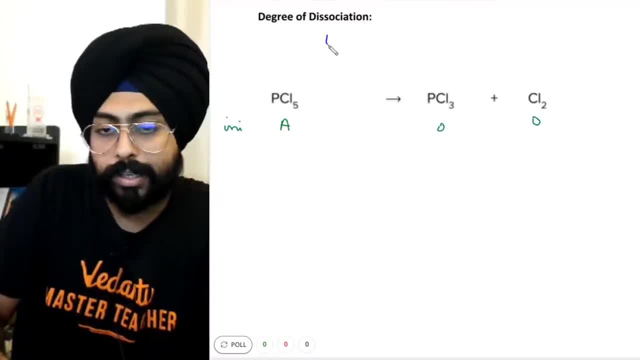 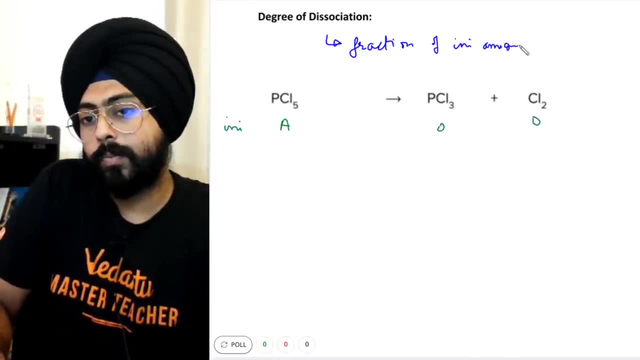 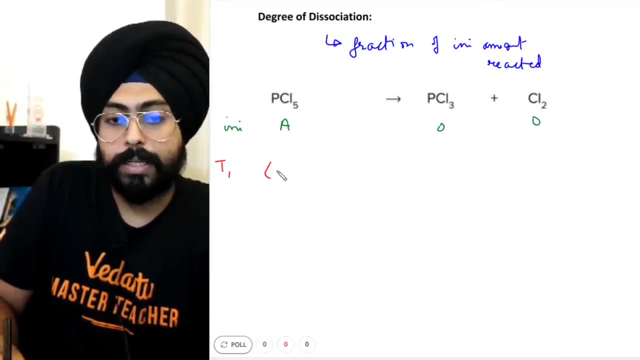 too complicated about it. so degree of dissociation- I will write over here once again- is just the fraction of initial amount reacted. as simple as that here at time. t1, this will be A into 1 minus alpha. this will be A into 1 minus alpha. this will be A into 1 minus. 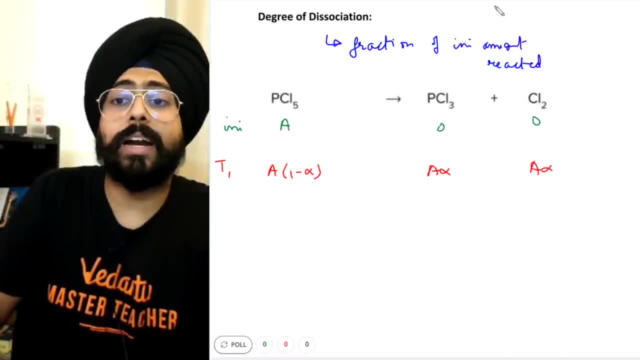 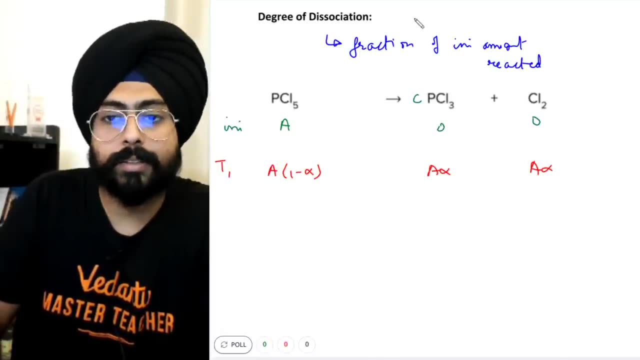 alpha, this will be A alpha. okay, if it had a stoichiometric coefficient, let's say C, then you will have C times A alpha over here. as simple as that. Okay, Great, there is nothing difficult about this, it's a very simple idea. degree of dissociation. 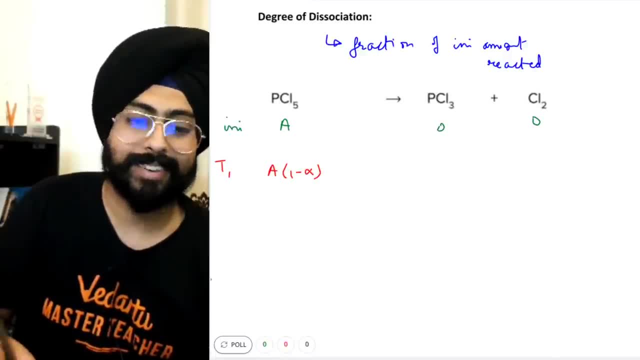 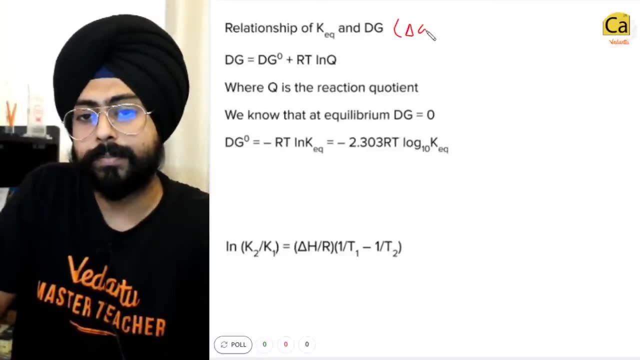 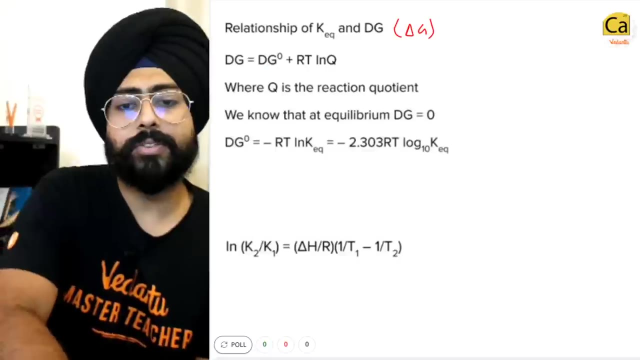 is the fraction of the initial amount that gets reacted. very simple. Now let's move on into relationship of K, equilibrium and DG. DG is essentially delta G, DG, delta G- same thing. okay, So delta G of a reaction is equal to delta G, naught. what is the difference between delta? 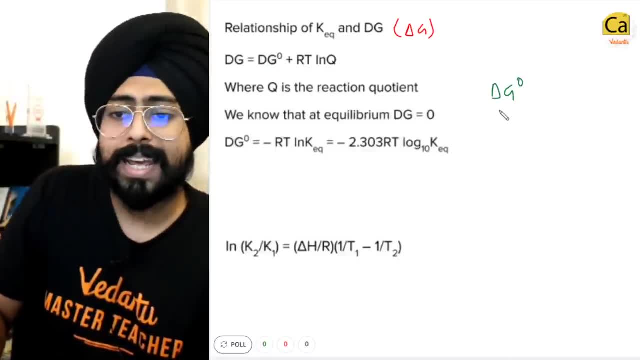 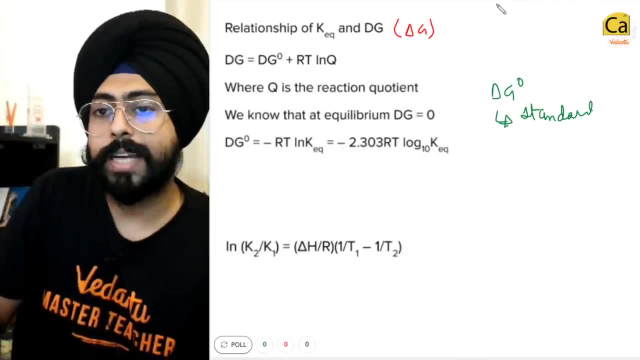 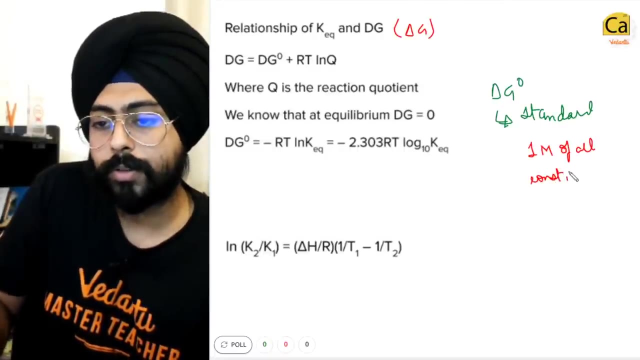 G and delta G naught, Delta G naught is at standard conditions. this is a standard, okay, this is a standard. so over here you have one mole of all constituents, okay, one mole of all constituents, one molar. 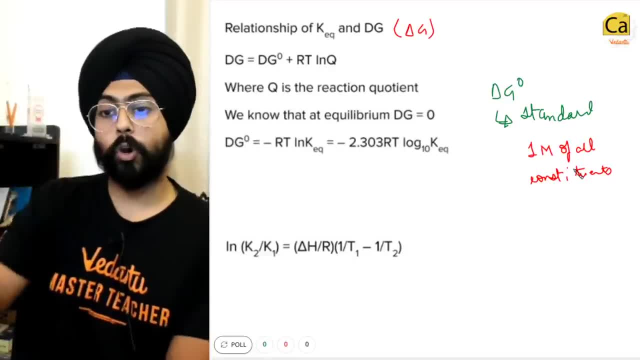 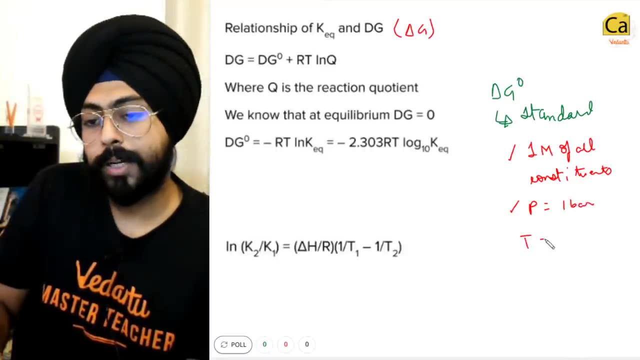 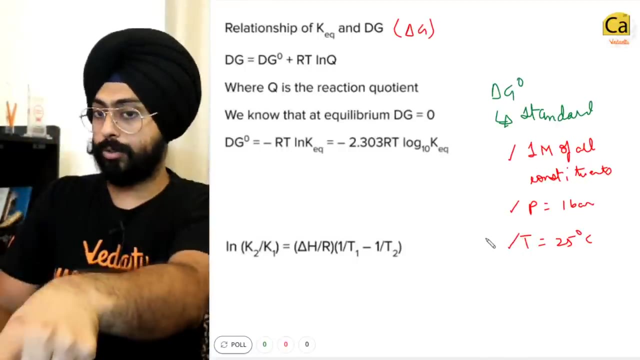 concentration: Okay, So reactants and products, all are one molar. to define delta G naught: okay, your pressure is equal to 1 bar, your temperature is equal to 25 degree Celsius. So delta G naught is delta G at standard conditions. how are they related to each other? 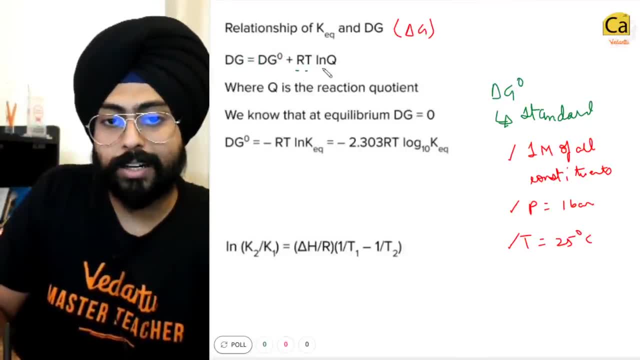 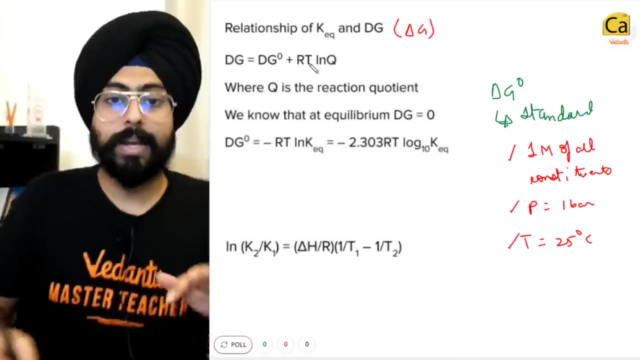 Delta G is equal to delta G, naught plus RT ln Q. okay, great, now all of us know that. at equilibrium, at equilibrium, Okay. So delta G is equal to zero. What is delta G? What is delta G? 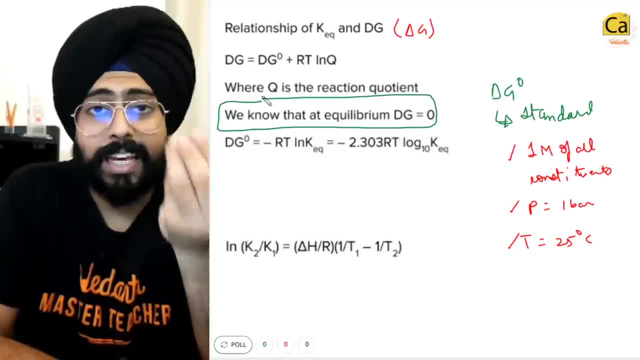 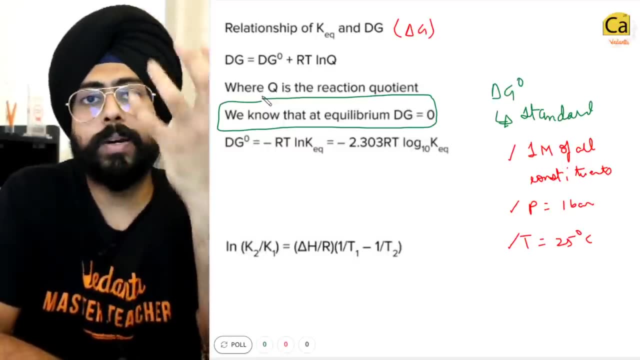 Delta is the delta. G is change in Gibbs free energy. what is Gibbs free energy? Gibbs free energy is the energy contained inside the system which it can use to do the reaction. that is why when delta G decreases, it means that the system has used its own. 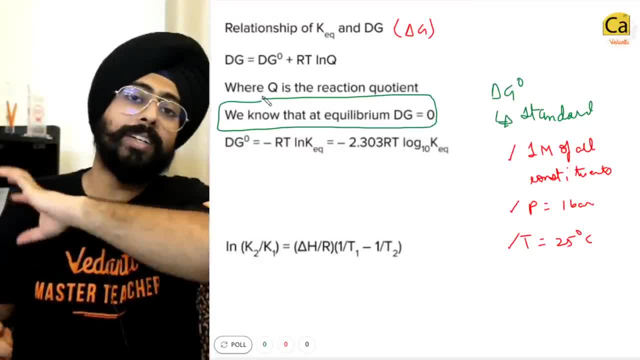 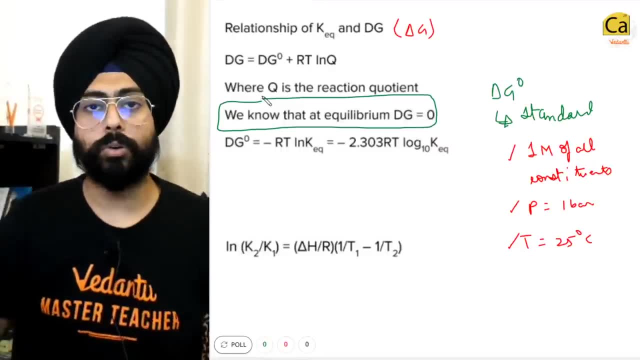 energy to do the reaction and once that happens, once it has used all energy, the reaction will stop happening, which means that all the energy has been used. now delta G is zero and equilibrium has come. when you are at equilibrium, the system is not using any more. 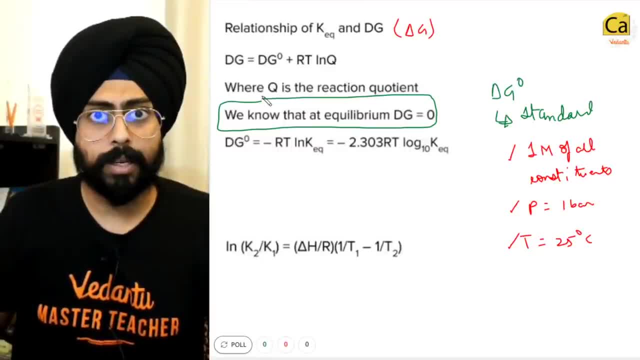 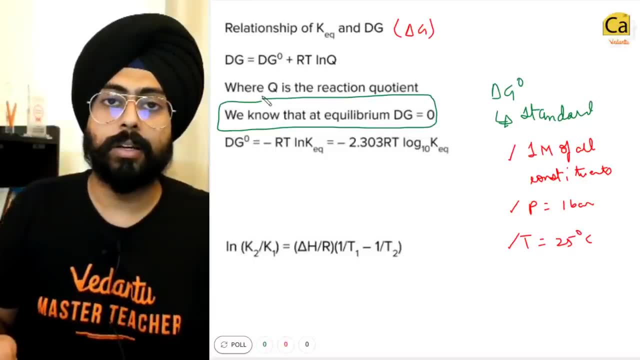 energy of its own to do the reaction. yeah, delta G Gibbs. free energy is the amount of non expansion work that the system is capable of doing, something that is an idea of thermodynamics. So over here, at equilibrium, since the system is not doing any more work, the change in 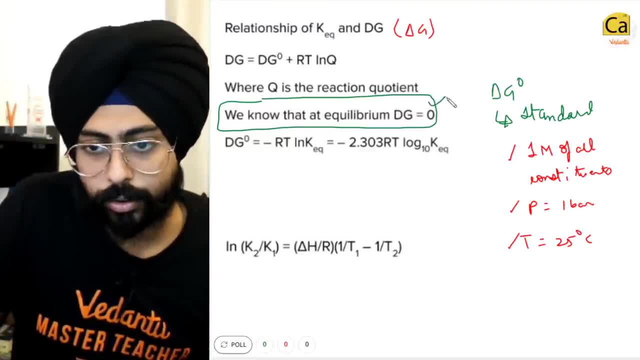 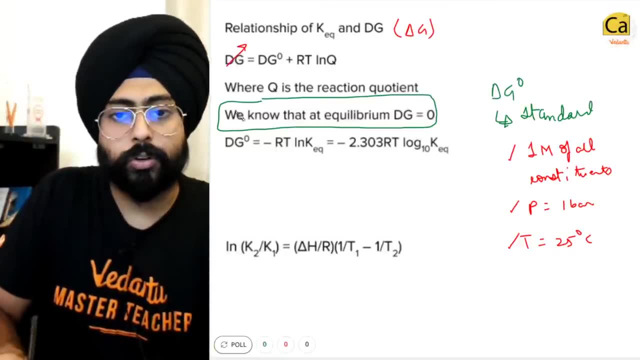 its own Gibbs. free energy is zero, So delta G is zero. But delta G, naught, is defined only at standard conditions, right? So if we put this guy equal to 0, we can get an expression between delta G0 and minus. 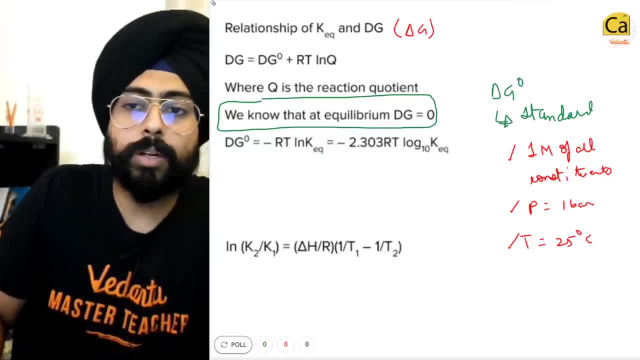 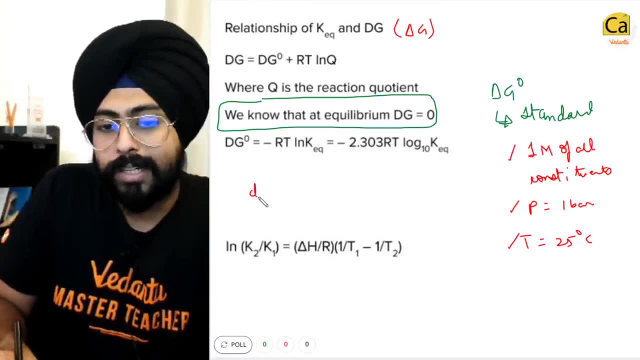 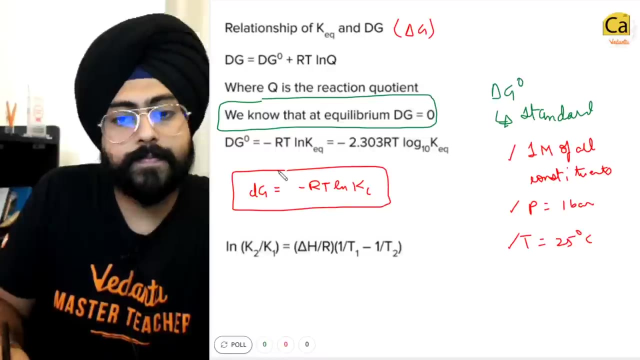 RT ln K equilibrium. why K equilibrium? Because reaction quotient will turn into K equilibrium at equilibrium. so you can write over here: DG is equal to minus RT ln Kc. fine, great. Then the other equation that I have given to you over here. of course, this is a revision. 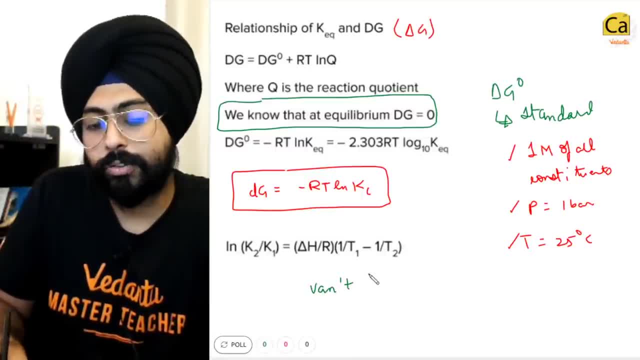 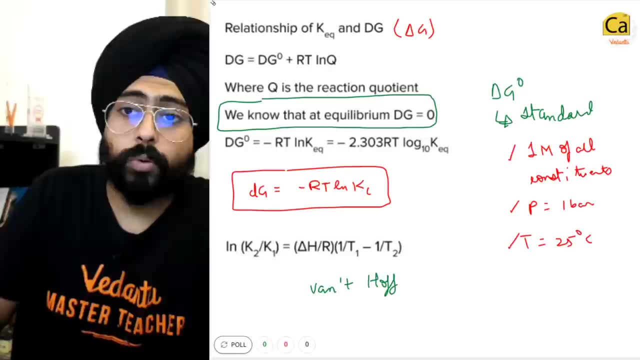 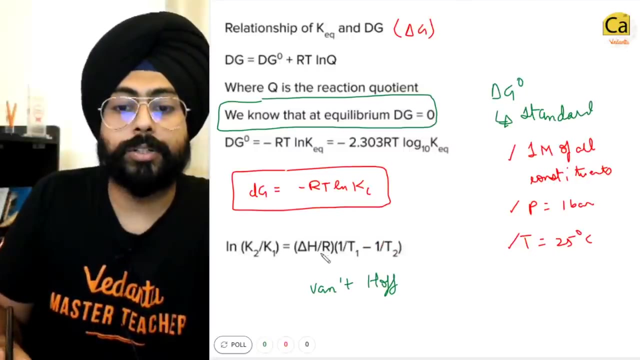 class. we won't be doing derivations. this is the Van't Hoff equation. I am pretty sure some of you have recognized this already. this is the Van't Hoff equation. what this does is it gives you a relationship between the equilibrium constants at different temperatures. 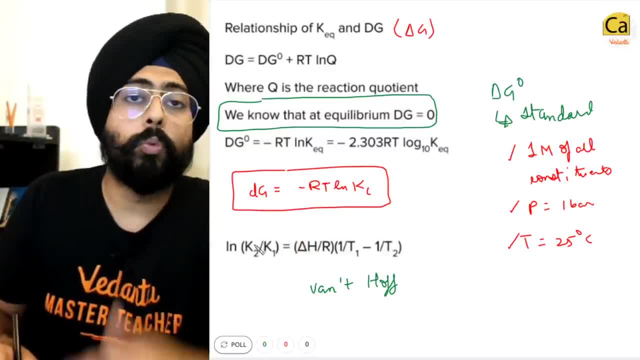 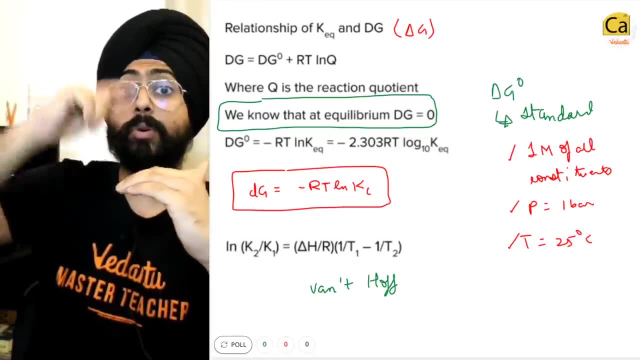 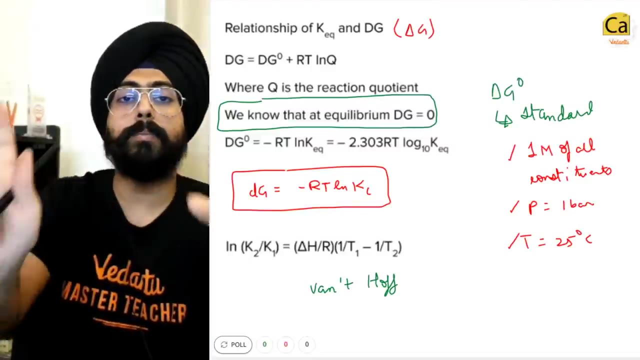 looking at just the enthalpy of the reaction. this can tell you what is the difference between the K equilibrium at different temperatures. do you realize? Do you remember that when you change temperature, K equilibrium changes? this is what the equation is quantifying. okay, K equilibrium will not change unless you change temperature. if you 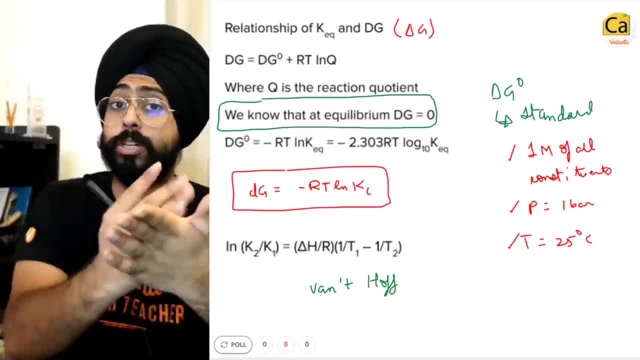 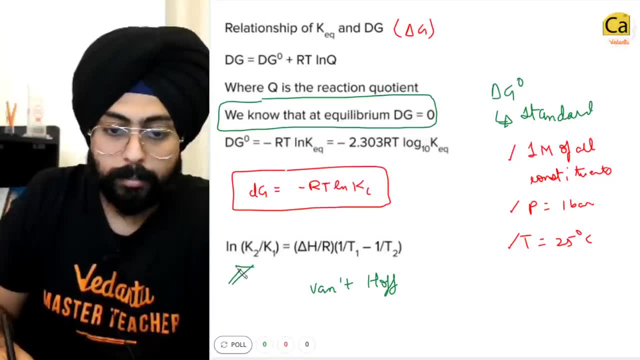 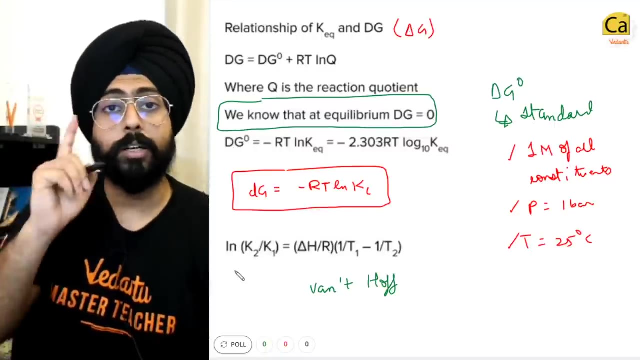 change, concentration, pressure, volume whatsoever- K equilibrium will remain constant, but if temperature changes, then your K equilibrium's value changes and those values are related to each other by the Van't Hoff equation. please remember this equation. this is important. we will use it in some question tomorrow when we are doing the question solving of this. 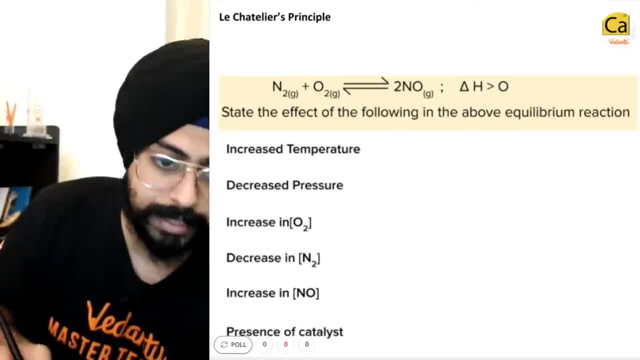 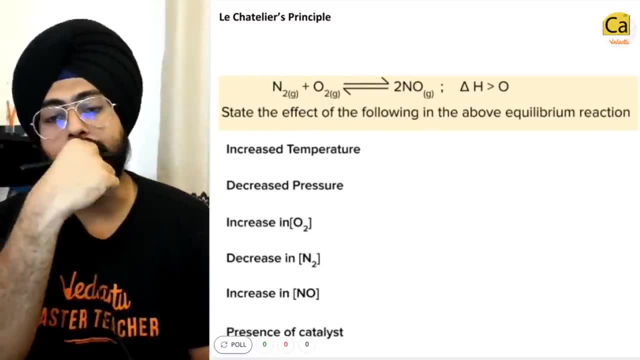 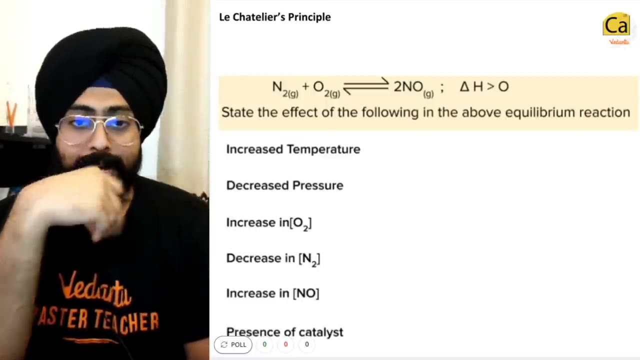 particular chapter at 8 pm. And now, my dear friends, finally, let's talk about Le Chatelier's principle. his actual pronunciation will be a very weird, something like that French pronunciation, I am not sure. let's call him Le Chatelier, for ease of use. Le Chatelier's principle tells us how, if we 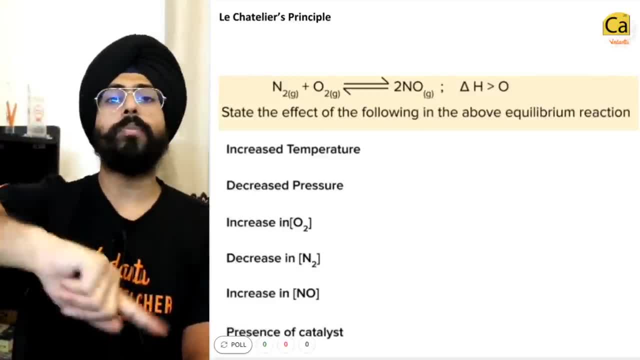 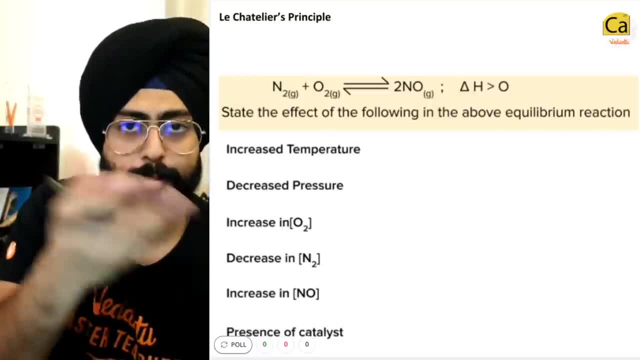 change different-different reaction conditions. reaction will go forward or backward, so on and so forth. yeah, fine, so let's do this with the help of an example. Let's make it a little more fun. state the effect of the following in the above equilibrium: 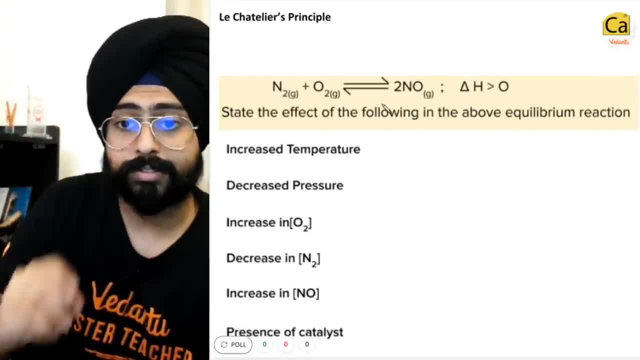 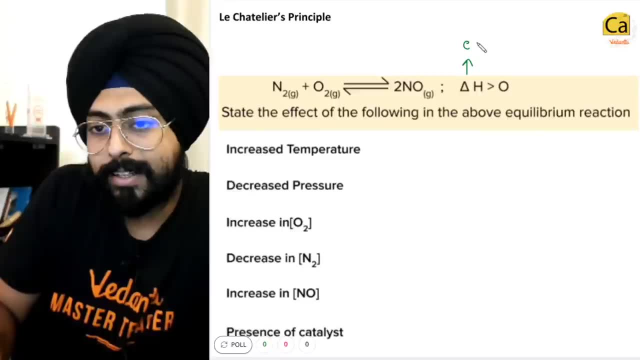 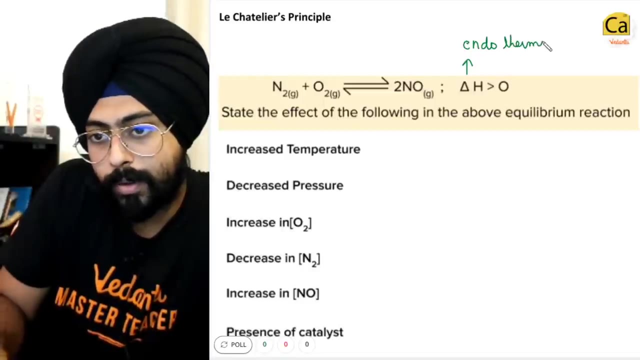 reaction over here. what are the facts of the reaction? let's try to understand the facts of the reaction. first of all, okay, delta H greater than zero. this means that this is an endothermic or exothermic reaction. this is an endothermic reaction because delta. 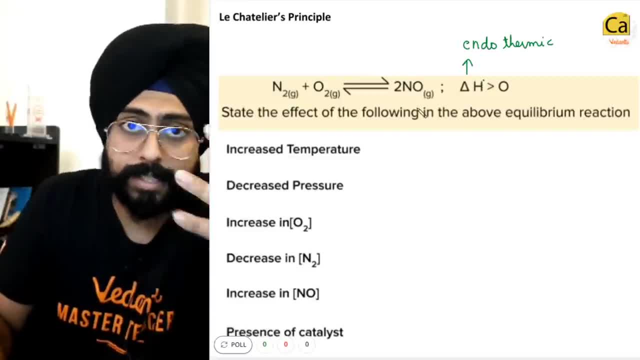 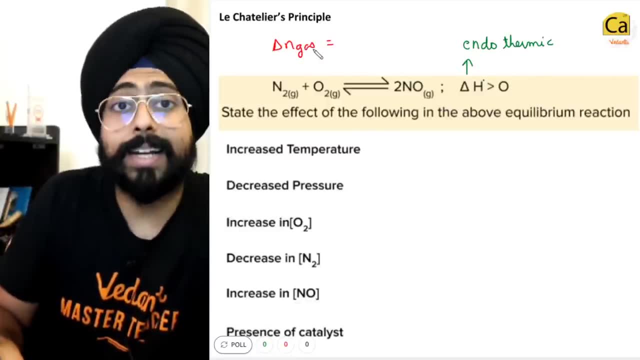 H is greater than zero, it needs heat. if delta H was less than zero, it was releasing heat Over here. what is the delta N gaseous? delta N gaseous is 2 minus 2, that is zero. yes. 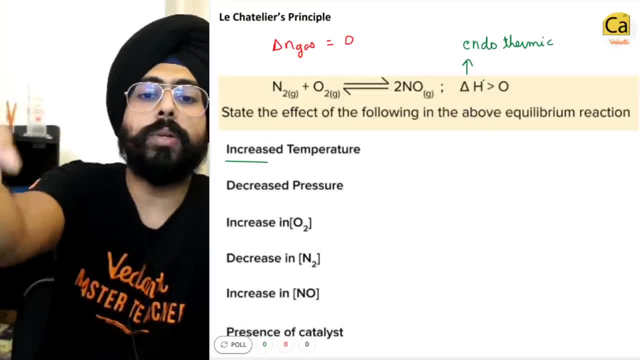 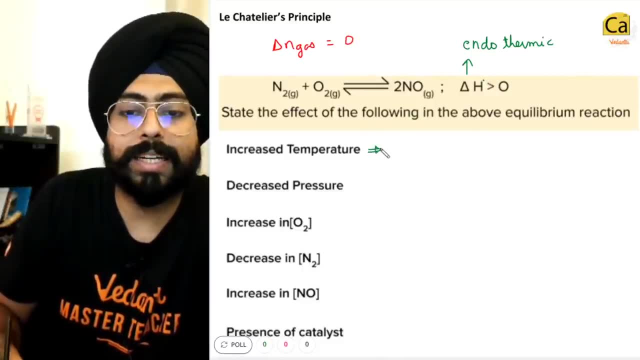 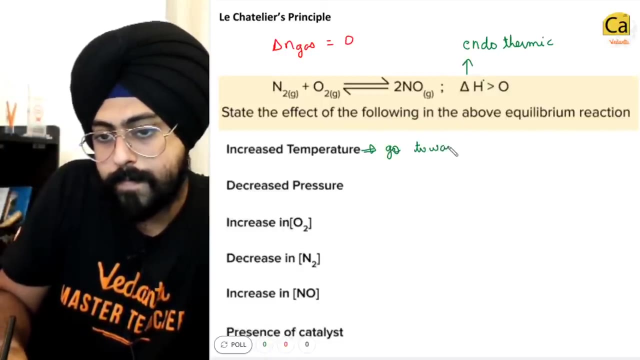 now people, let us revise all of these points and also see what will happen in the case of this particular reaction. what is the effect of increased temperature? what is the effect of increased temperature? increasing temperature implies that you go towards, go towards, okay. 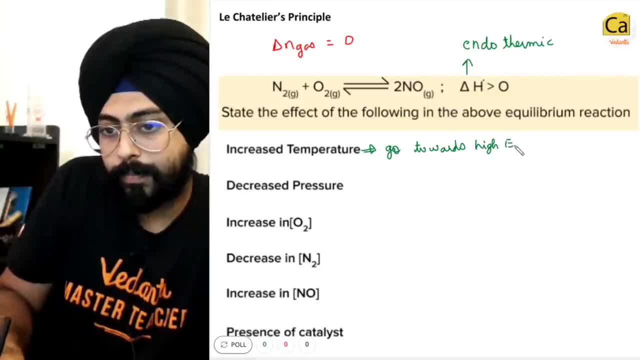 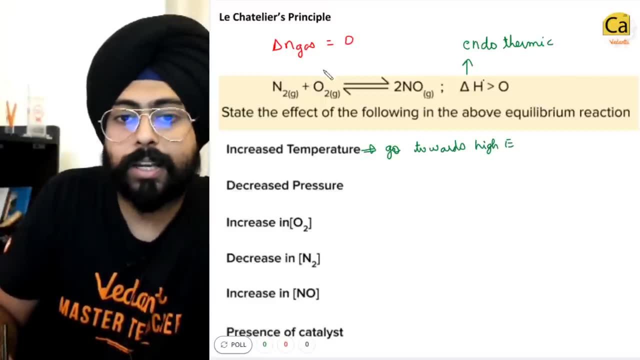 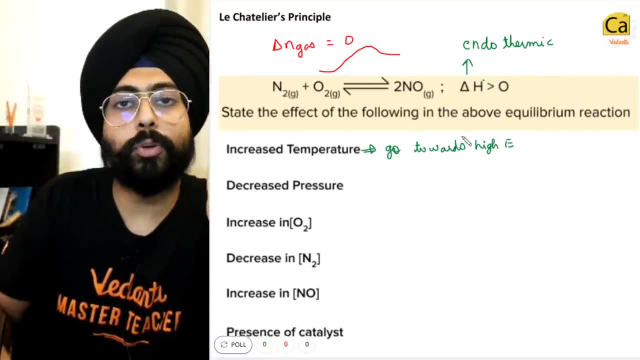 one second: go towards higher energy. since this is an endothermic reaction, do you realize that the reactants are at smaller energy than the products? the products are at higher energy, so you increase temperature. you have to go towards higher energy. so over here in this. 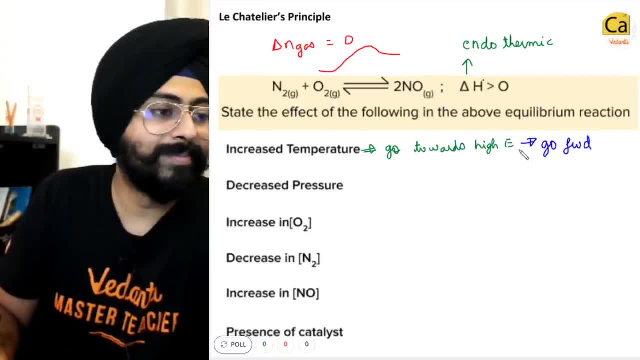 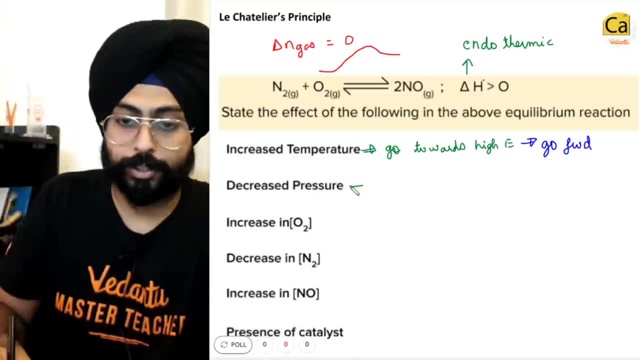 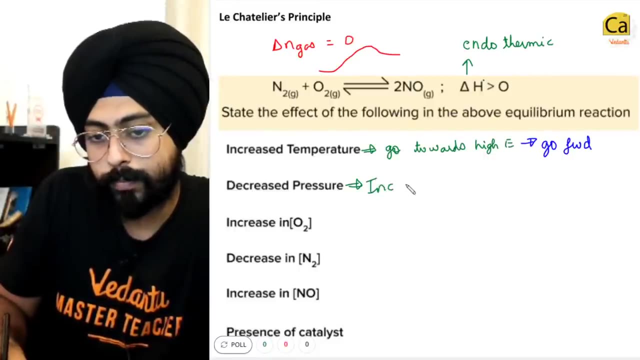 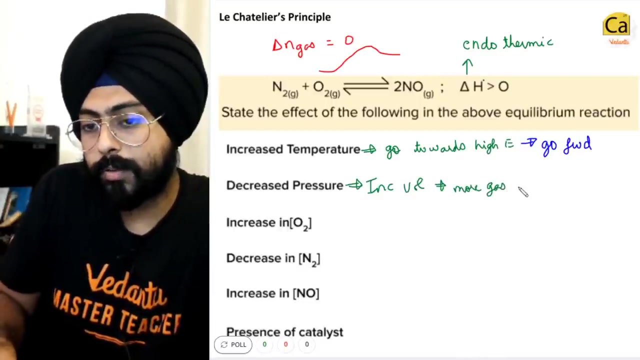 reaction: you go forward, you go forward. what if you decrease pressure? okay, if you decrease pressure, you can assume. okay, if you decrease pressure, you can assume that is an increase in the volume. If you increase the volume, it has to go towards more number of gaseous moles. yeah, if you. 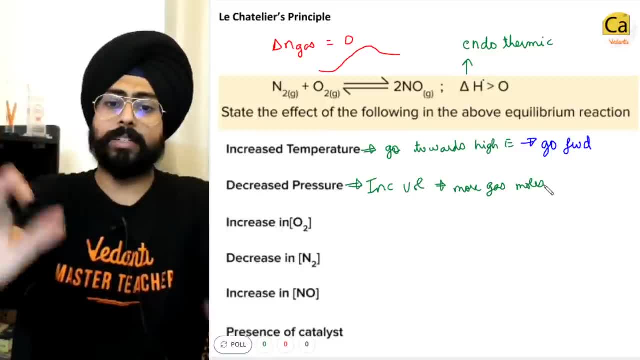 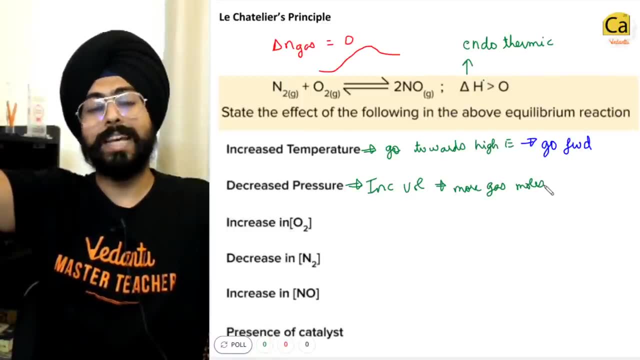 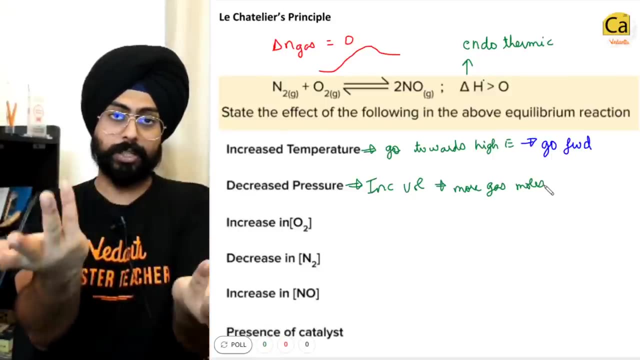 decrease pressure, you can imagine that the volume is increasing. that is how you can imagine. if it is a constant volume system, then no change will happen. If volume increases, the system goes towards more number of gaseous moles. if the volume decreases, the system goes towards less number of gaseous moles. Over here in the reaction. 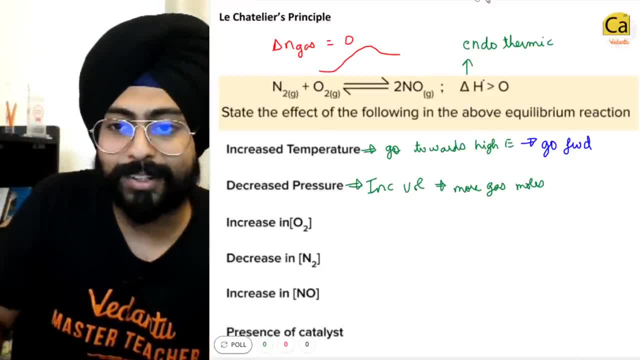 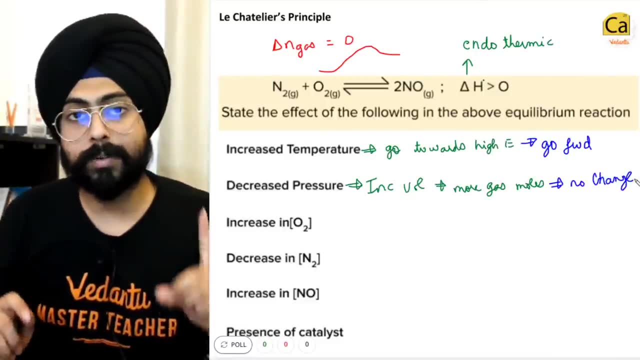 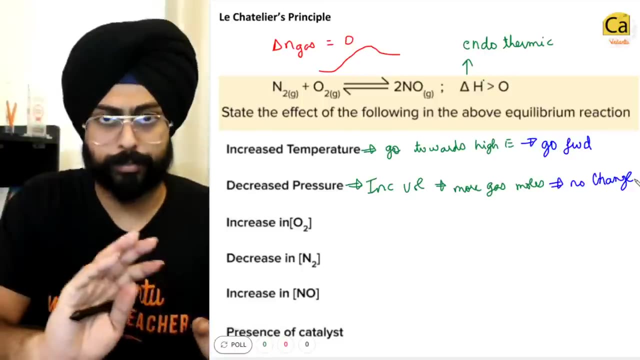 there is no change in the number of gaseous moles, so this particular reaction has no change by the change in pressure or volume. Always remember: volume change dictates the change. If you have an isochoric vessel and you change the pressure, no change will happen, Only if 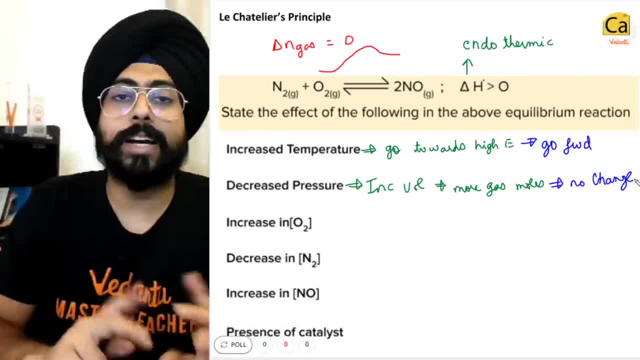 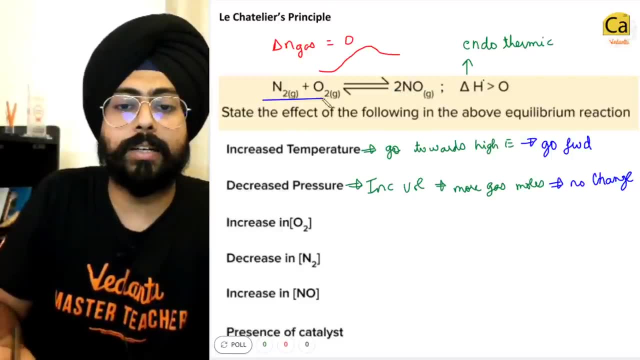 pressure can change volume, then your reaction might go forward or backward depending on the delta N Over here. since delta N is zero, gaseous moles on the right hand side are two. gaseous moles on the left hand side are two. no change, Then increase in concentration. 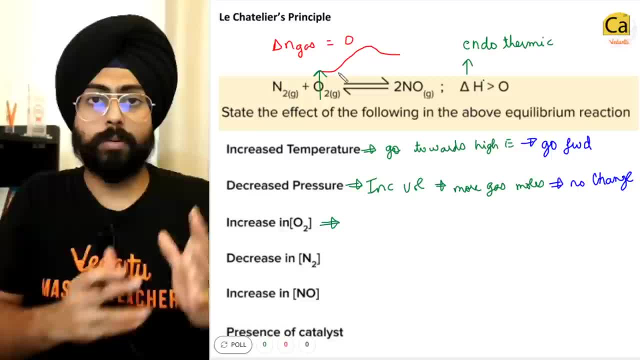 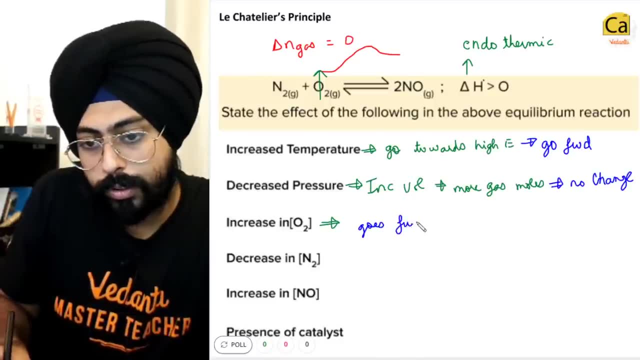 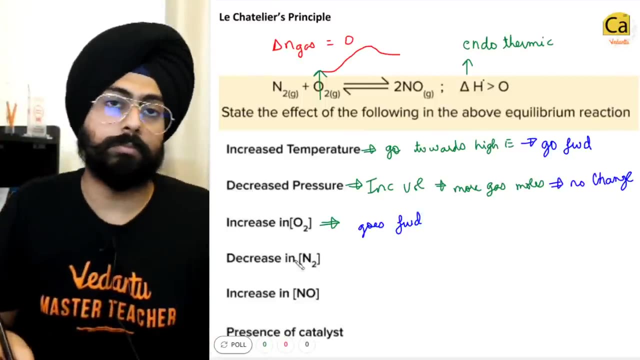 of O2, reactants are increased. more reactants, more opportunity to react. it will go towards the product. It goes forward, isn't it? Reaction ho raha hai, reaction ho raha hai. Suddenly, the reactant increases. let's go towards the products. Simple as that. N2 increases. 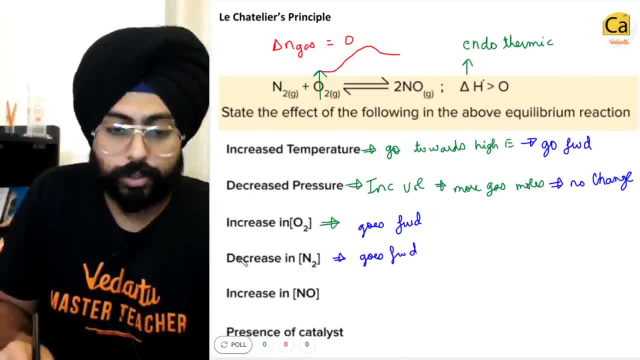 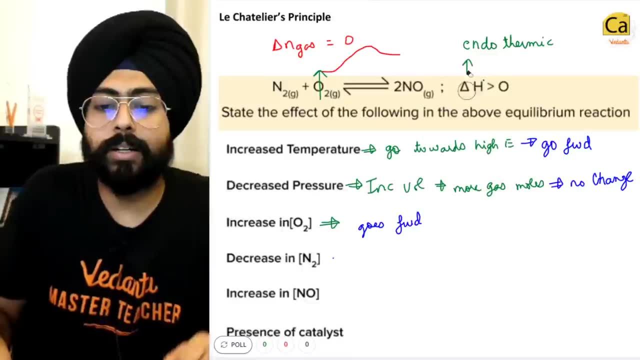 once again goes forward. Okay, sorry, yaha, par decrease, likha hai N2 decreases, So you are decreasing the reactants. So you are like: oh, I don't have enough reactant, make more reactant, please. So the reaction over here. what will happen to the reaction? The reaction. 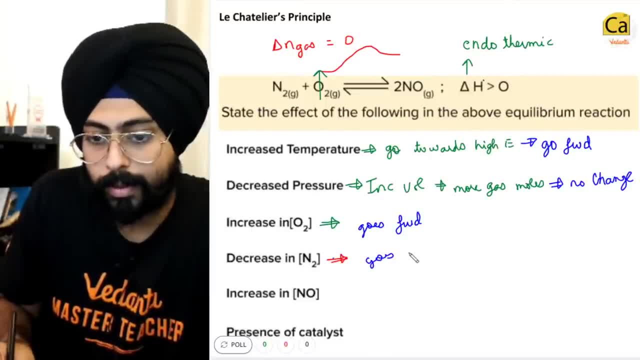 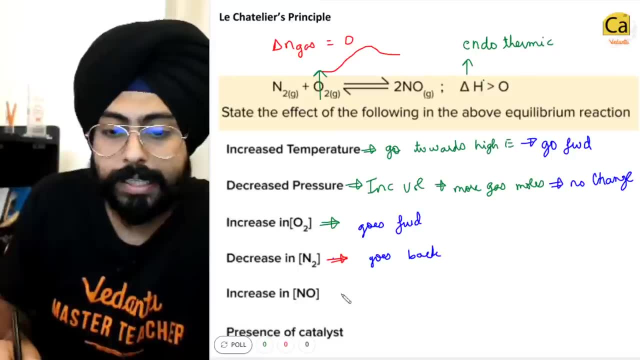 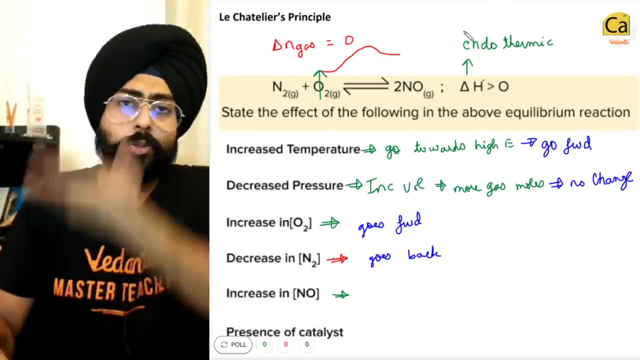 will go backward. goes back. Similarly, if you increase the reactant, the reaction will increase the anode concentration. if you increase the products concentration, lots of products formed. the reaction will come back to the reactants. Very logical idea is: jo zada ho gaya usko kum kar dena hai. jo kum honge usko zada ko karn identification. 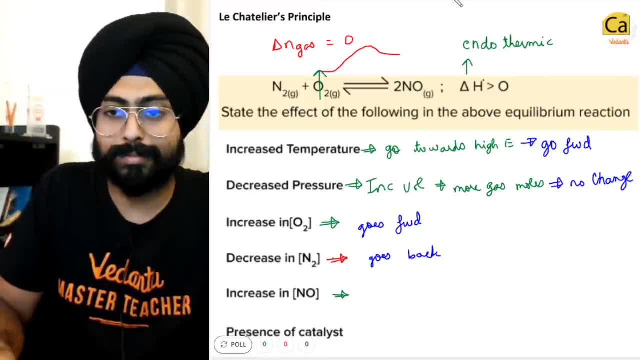 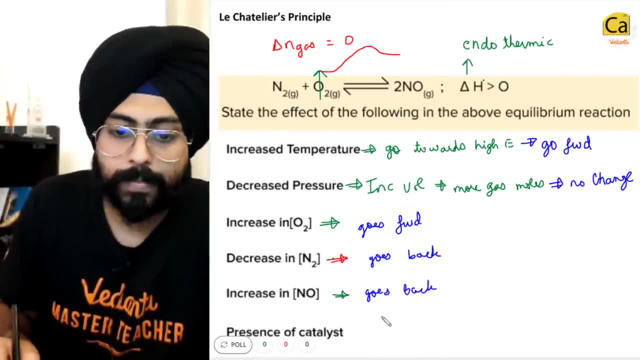 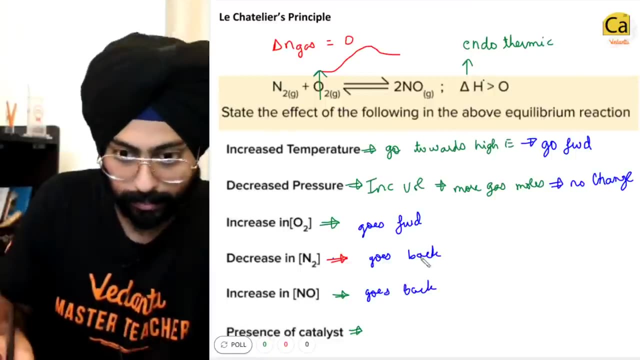 hai, if something increases, decrease it. if something decreases, increase it. as simple as that. So increases no, increases no goes back. Presence of catalyst. as we all know, catalyst does not change the reaction conditions at all. In the presence of catalyst, they urgent, they also change In that specific case you. 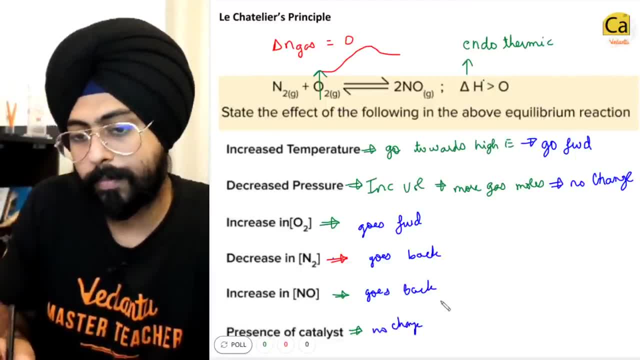 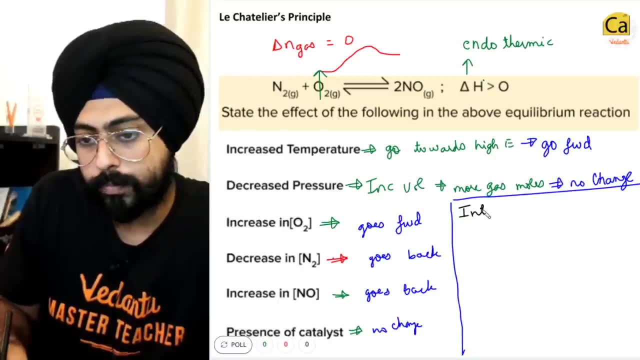 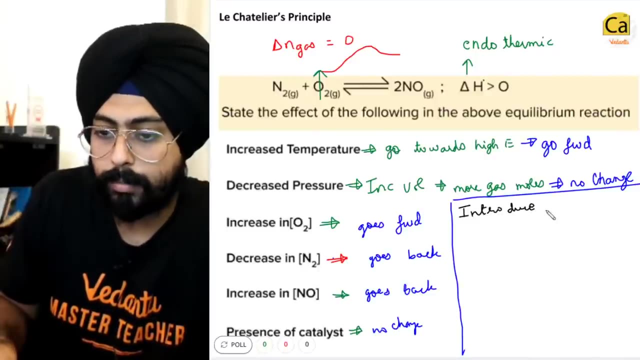 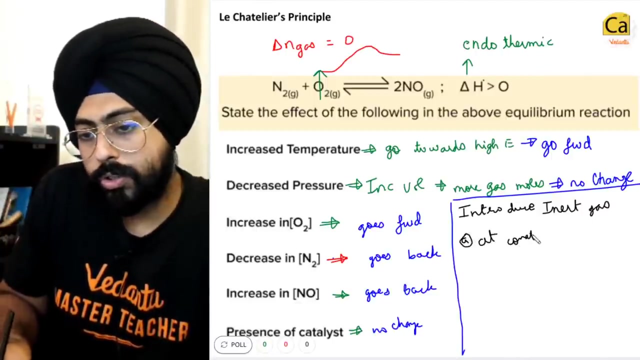 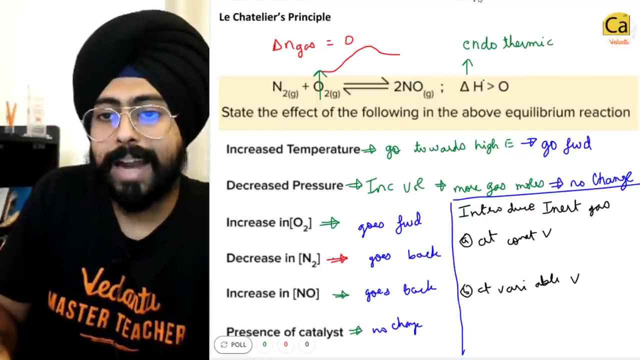 presence of catalyst, no change will happen. Two more cases that we will discuss quickly and our revision is over. Introduce inert gas At constant volume. at variable volume, At constant volume, my dear friends, at constant volume. if you introduce inert gas volume, 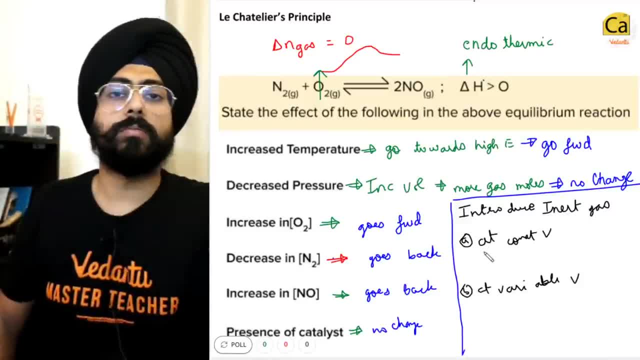 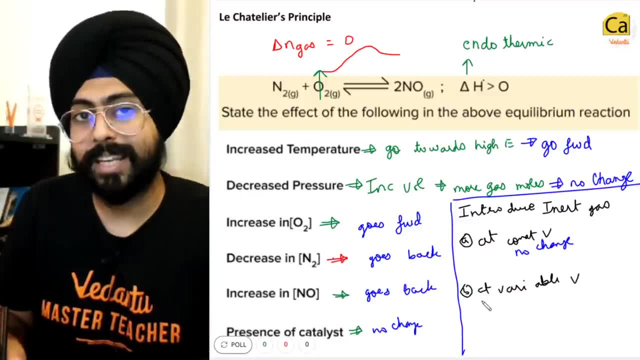 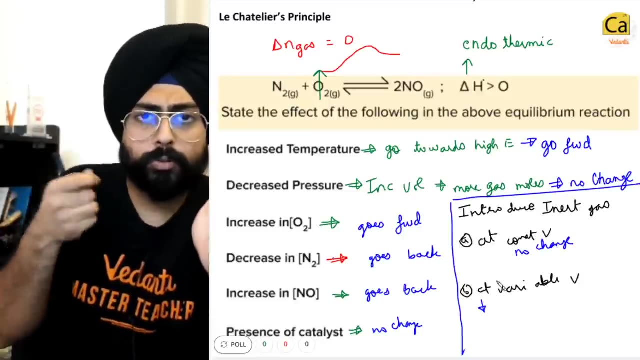 is not changing, Since the volume does not change. no change will happen In the case of variable volume. now what is happening? If you introduce inert gas, volume will increase. It's like a balloon: If you put more gas into it, it will increase. So for variable volume, 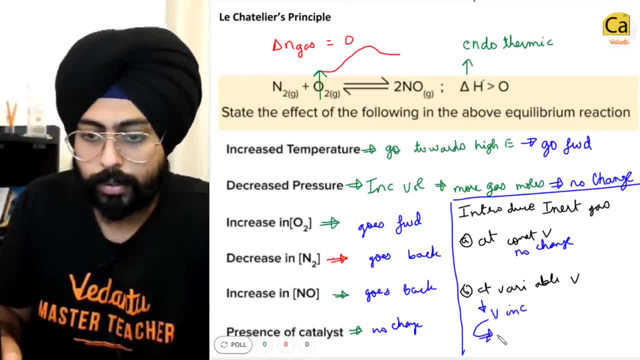 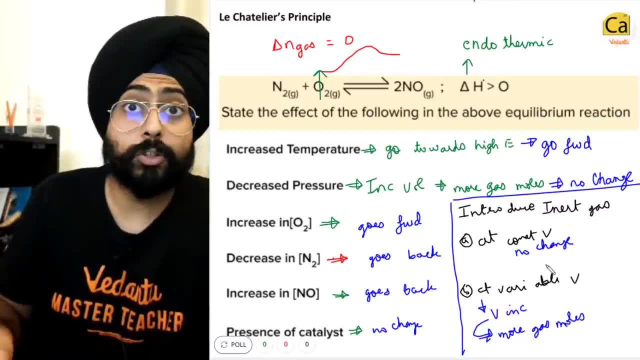 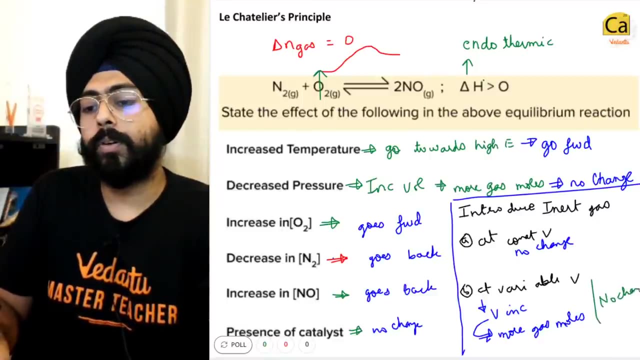 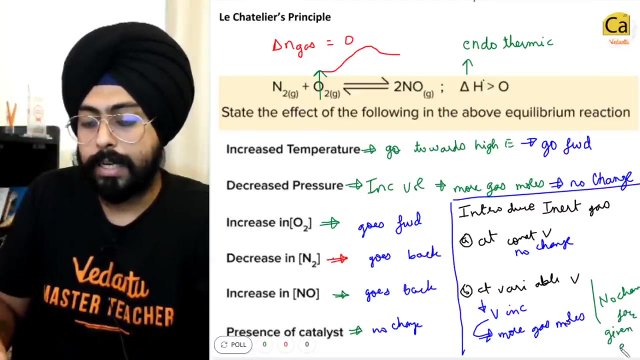 volume increases, This has to go towards. this goes towards more gaseous moles, isn't it? If you increase the volume, the system has to go towards more gaseous moles. But in this particular reaction over here, there is no change. No change for the given example. As simple as that. 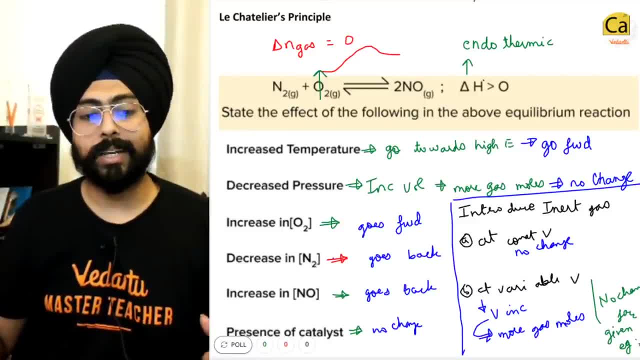 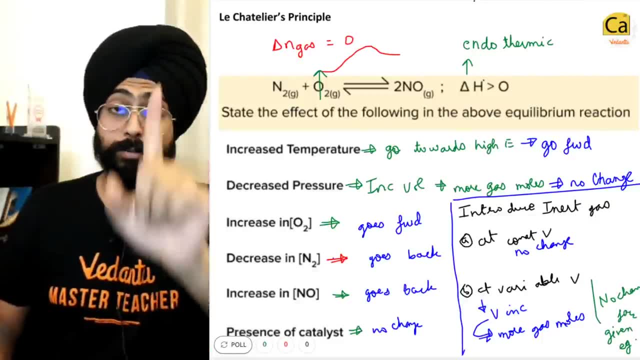 Lesch-Atelier's principle revised. Hardly took us any time. So, my dear friends, these were all the ideas that are there in the chemical equilibrium chapter. Very easy ideas, but the weightage of this chapter is important. This chapter finds its weightage almost every year in the examinations. 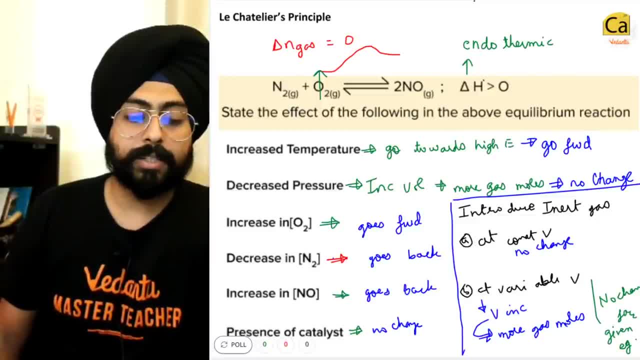 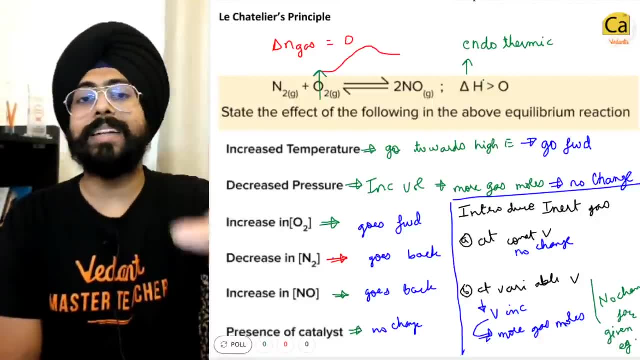 One question comes from it in high" uIn advance. Sometimes it does, Sometimes it does, And this chapter forms the basis of the ionic equilibrium chapter. Ionic equilibrium is pension Moynix. ionic equilibrium is just a fancy application of Lesch-Atelier's principal. 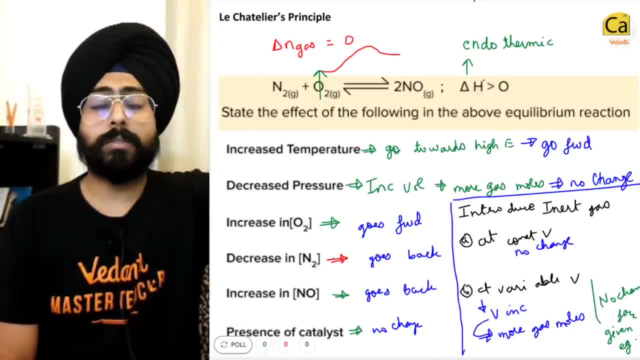 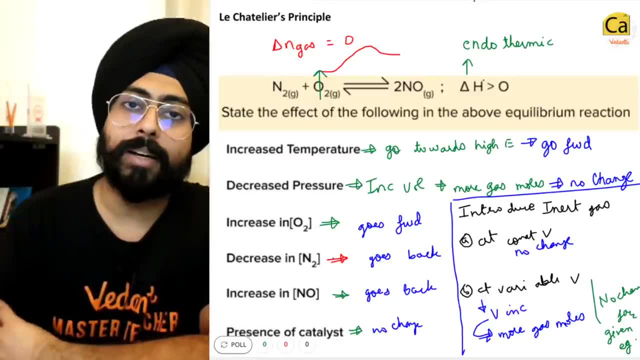 Common ion, in effect Lesch-Atelier's Principle- Certainly, we are seeing the inquiry with海centara Bye principle: pH varying in the condition of small acids, big acids, this and that it's all. Le Chatelier's principle applied in a mathematical fashion. okay, so ionic equilibrium. 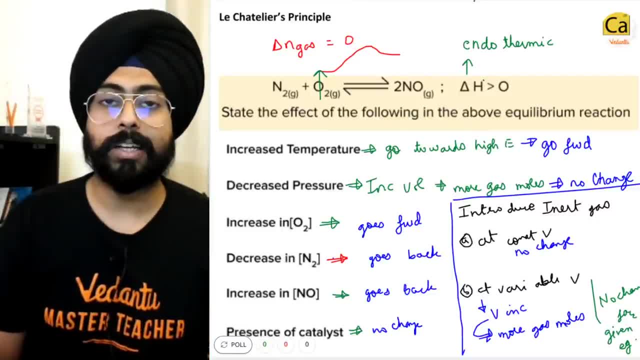 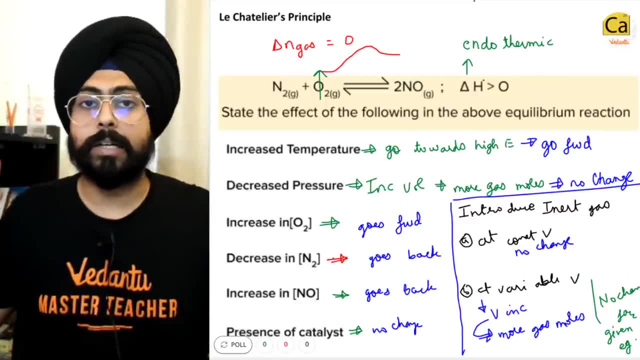 will be discussed in the month of June. please stay subscribed to the channel in case you don't want to miss that. alright, and in case this revision was helpful for you, please make sure you hit that like button. we are done. revising the chapter of chemical equilibrium. 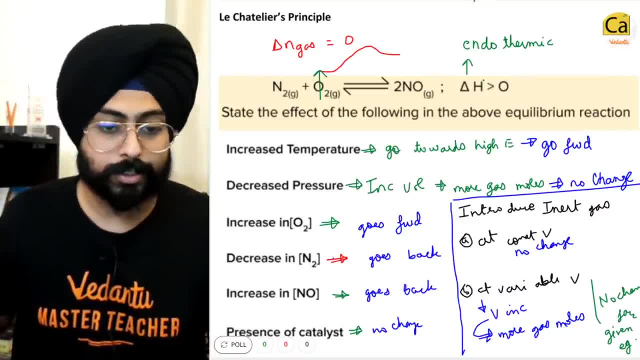 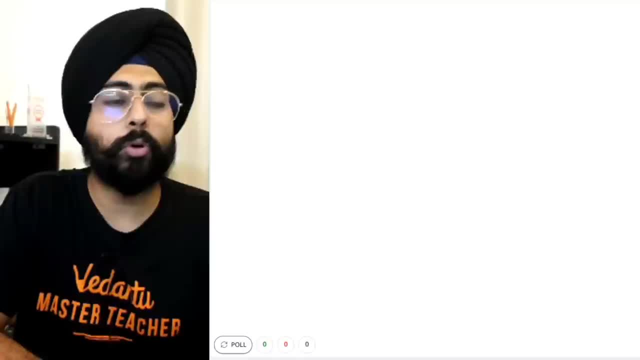 in just 30 minutes and we went into a lot of detail as well, so that's good. so, in case you enjoyed the class, make sure you hit the like button, stay subscribed and, for those of you who are asking questions, questions will happen tomorrow at 8pm.